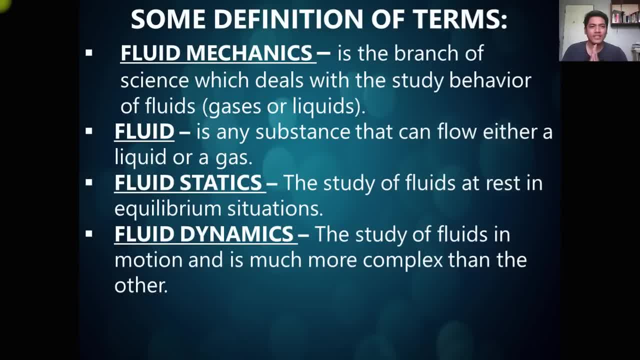 So let us start with some definition of terms. What is fluid mechanics? Fluid mechanics is basically the branch of science which deals with the study and the behavior of fluids such as gases or liquids. The misconception all about fluids is that when we talk about fluids, the first thing that comes to our mind is that fluid is limited to a liquid form. 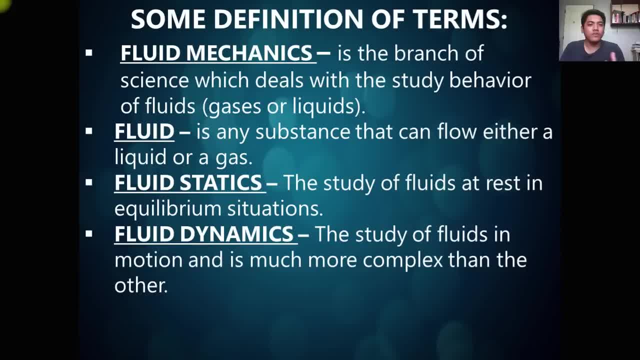 But in the case of the study of fluid mechanics, fluid is not only in liquid form, But basically a fluid is any substance that can flow, either a liquid or a gas, Meaning to say, even a gas can be considered as fluid. Why? Because it can flow. 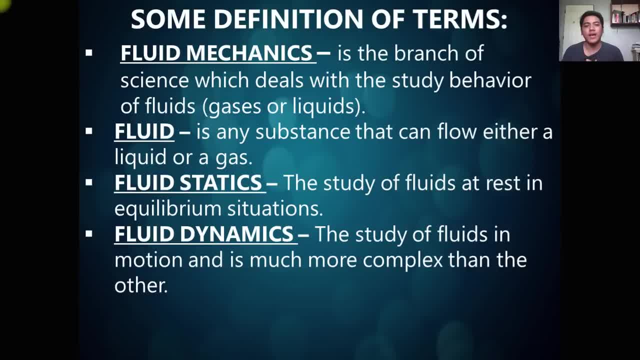 So in the study of fluid, that is the basic definition of fluid mechanics. So we have two branches of fluid mechanics And we have the fluid statics, which is the study of fluids at rest, meaning the fluid is not moving, Okay, it's just resting. 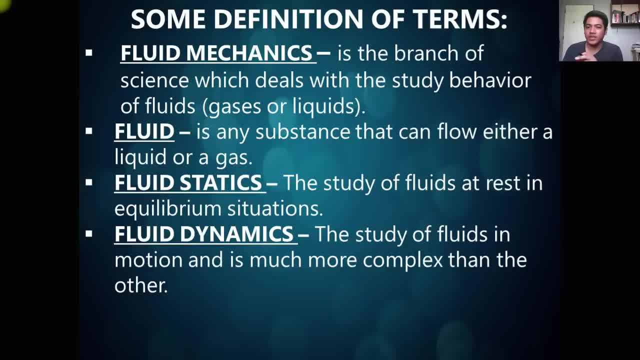 So the magnitude of forces acting along the fluid is zero because it is at rest- Rest in equilibrium situations- And we have the fluid dynamics. Once this fluid starts to move, then we are talking about fluid dynamics here, And this fluid dynamics is much way more complicated or complex than the fluid statics, because now the fluid is now moving. 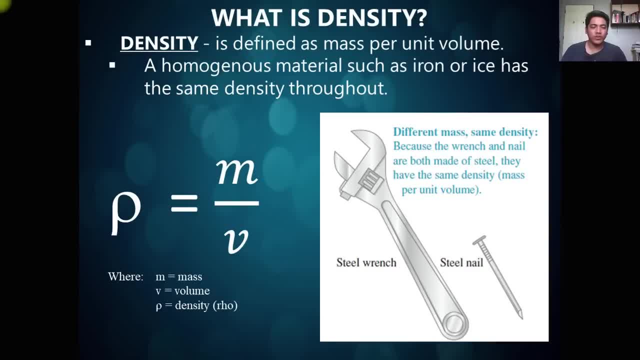 Okay, so here is some important quantities When talking about fluid mechanics. so we have what we call the density of the material. So what is this density? Basically, density is defined as the mass per unit volume. Okay, so it is basically represented by a Greek alphabet, Rho, and that is equivalent to mass of the substance over the volume of the substance. 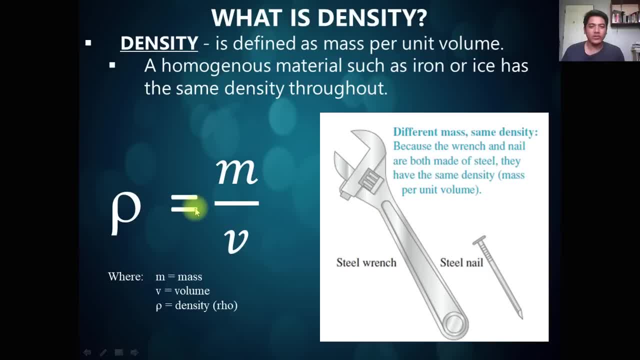 Okay, wherein our unit for density is SI, unit is kilogram per cubic meter, because volume is cubic. Okay, a homogeneous material, that is, a material that has the same material, Composition of material, has the same density. In other words, for example, we have a same. 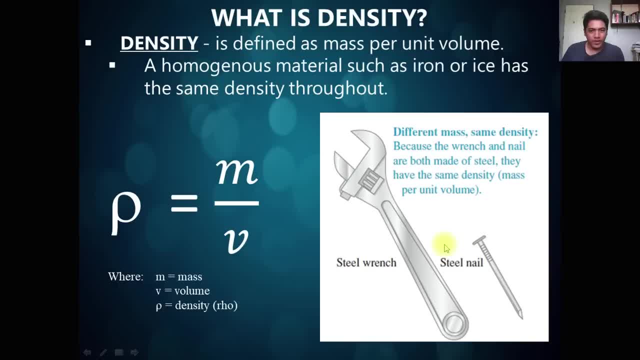 Steel wrench here and steel nail. They are both steel, Though they have different shape and different mass. Okay, their density is the same Because they are a homogeneous material. They are composed of the same material. So different mass, same density for steel wrench and steel nail, regardless of their size and regardless of their 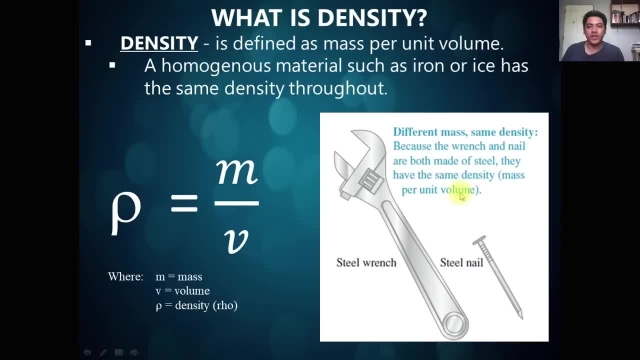 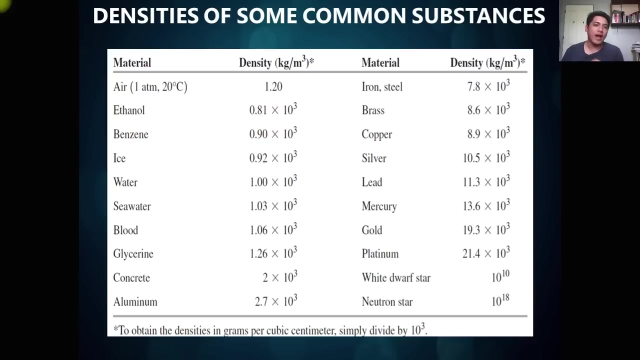 mass. So because the wrench and nail are both made of steel, they have the same density: mass per unit volume. And again, density is an important parameter on whether the object would actually sink or float. Okay, when submerged into a liquid, Okay, so density, that is basically density. So here are some densities of some common substances We have. 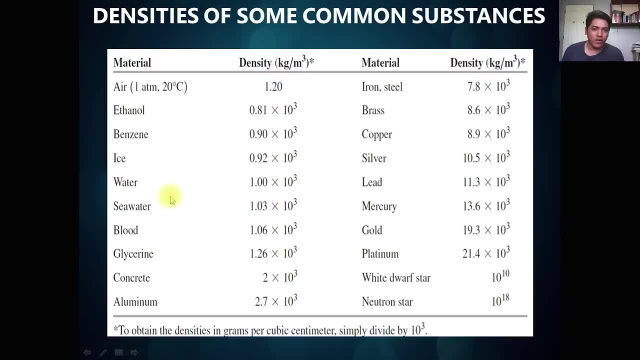 The most common is water, Wherein the density of water is 1 times 10, raised to 3 kilogram per cubic meter. So that is the density of water. for every element, we have the density, the constant density. Okay, so Do we need to memorize all of this? Not necessarily. 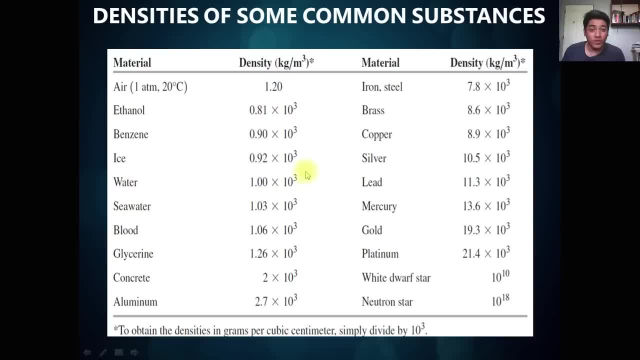 but we have to take note what is the density of water, because sometimes in the problem it's not given. So that is basically 1 times 10, raised to 3 kilogram per cubic meter, And we have the air: 1.2 kilogram per cubic meter. 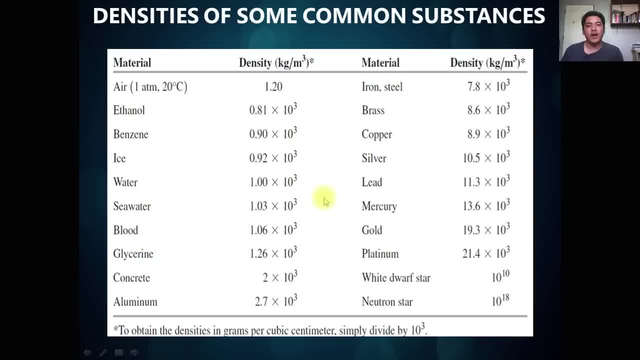 We have the ethanol, the benzene, the ice and different elements here. Okay, so, we have the densities of some common materials. Okay, so, let's try to solve a problem. Okay so, let's try to solve a problem. Okay, I've written the problem here. 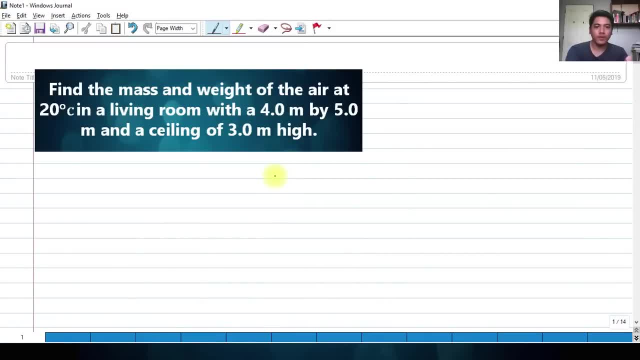 So for our problem number one, Find the mass and weight of the air at 20 degrees Celsius, that is in Celsius, in a living room with a 4 meters by 5 meters in a ceiling of 3 meters high. So basically, we're asked to find the 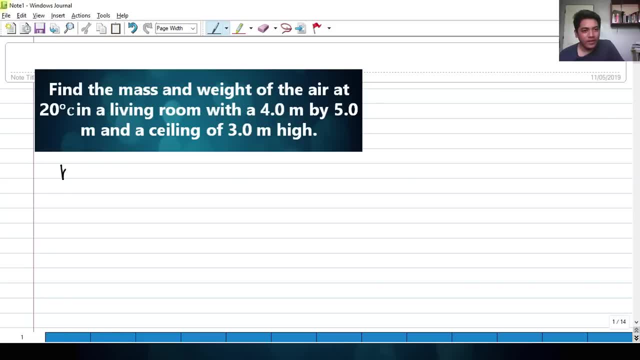 mass of the air and the weight of the air inside the room. So what is the mass of the air? What is the weight of that air? Okay, using the formula- density is equals to mass over volume- We can calculate the air, the mass of the air inside the room. 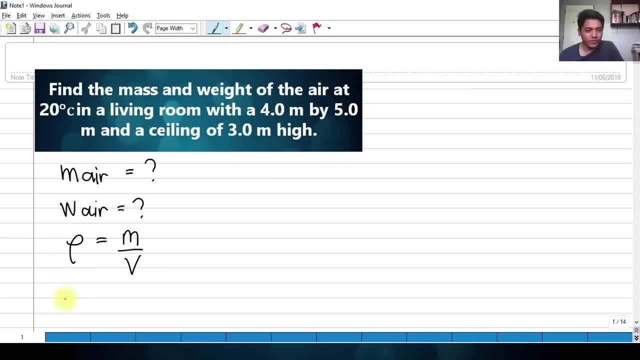 So, of course, inside the room we have, the density of air is equals to the mass of air divided by the volume of the room. Okay, so what are we going to do? So what we're going to do is to get the mass of the air. simply we cross, multiply that. 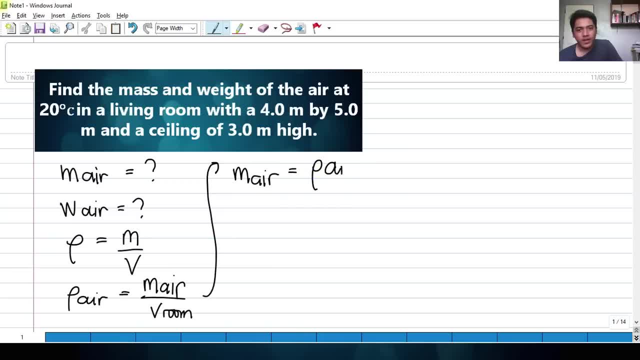 Okay, mass of the air is simply density of the air times the volume of the room. Okay, so the density of air is shown a while ago- 1.2 kilograms per cubic meter- and the volume of the room is that. that is a cube. 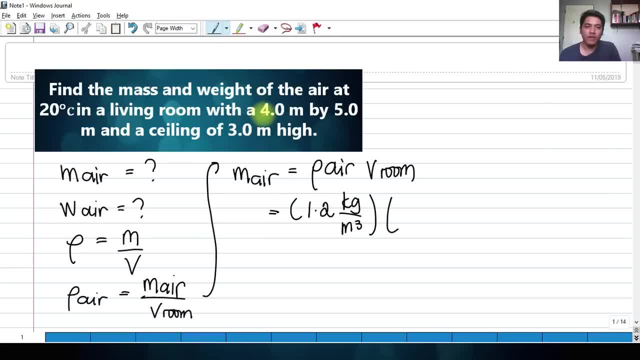 So because we have not a cube necessarily, so we have a 4 meter by 5 meter by 3 meters. So we have a 4 meter by 5 meter by 3 meters. So length times width times, height of the room, so we have 4 meters. 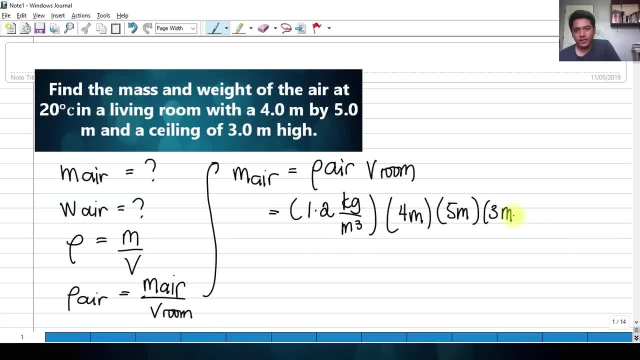 multiplied by 5 meters, multiplied by 3 meters, okay, and this should give us this meter- cubic meter will cancel, okay, And that should give us 72 kilograms, if I'm not mistaken. so let's try to verify. So 72 kilograms, that is the mass of the air inside. 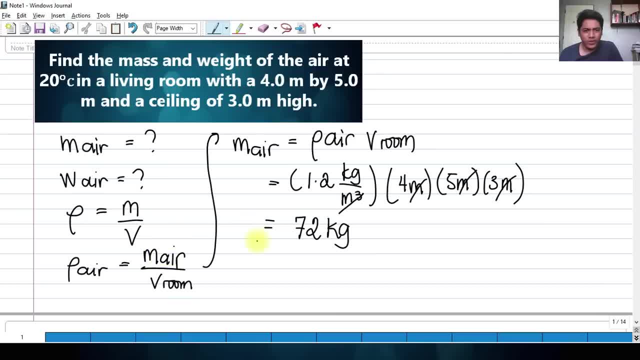 that room. How about the weight of the air? Well, actually we know that the weight of the air is simply the mass times the acceleration due to gravity. that is 72 kilograms multiplied by 9.81 meter per second squared, and weight should be Newton. So that is 72 times 9.81.. That should be 706. 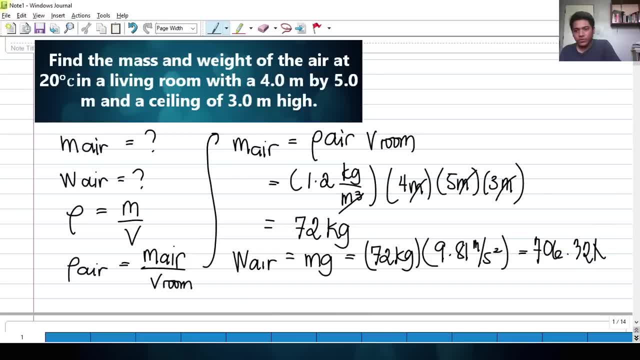 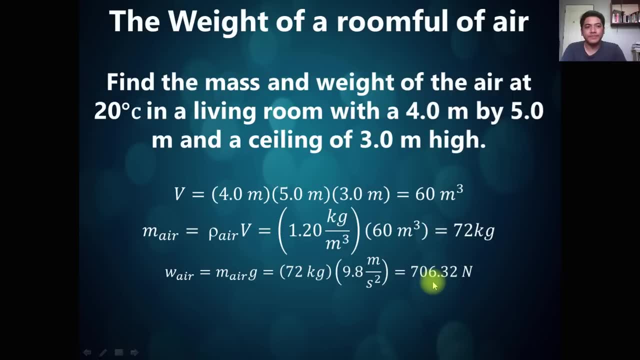 706.33, 706.332, 706.332, 706.332, 706.332. That should be our answer for the weight and the mass of the air. Okay, so this is our computation. okay, We have the same answer. okay, So how about? pressure Pressure is also an important 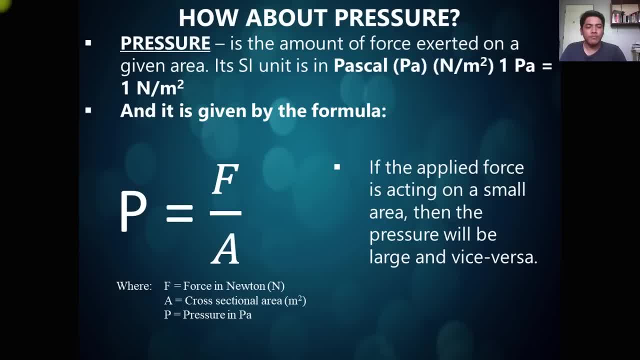 quantity when we are talking about fluid mechanics and pressures, basically defined as the amount of force exerted on a given area. This force is actually perpendicular to the normal or the surface area of the object. okay, So, and its SI unit is given in Pascal. okay, 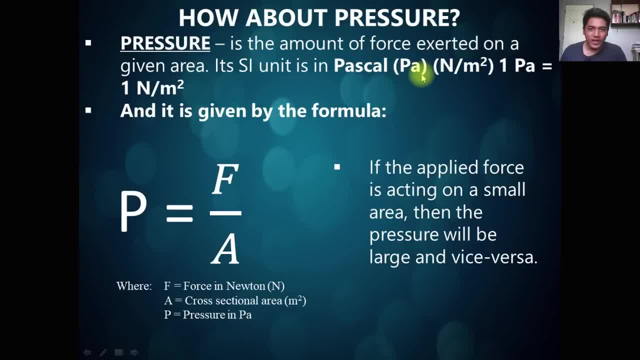 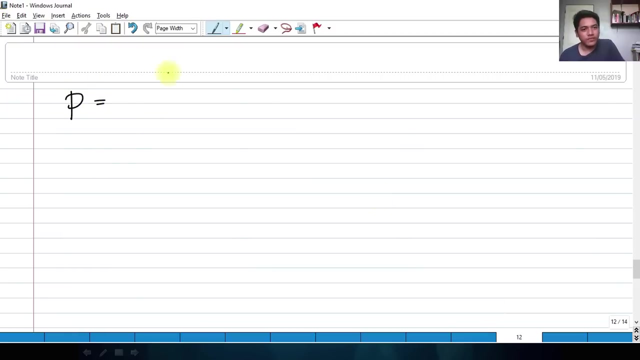 And Pascal is denoted by PA And of course the unit of pressure is denoted by 1 newton meter per meter squared, It's actually equal to 1 Pascal. So in other words, if we're going to write the pressure equation, so pressure is defined as the force per unit area. 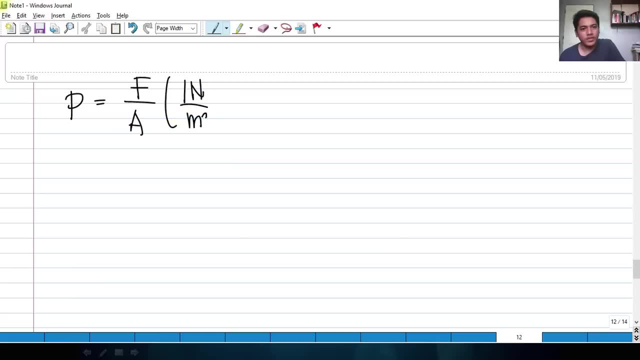 And the unit of force is actually 1 newton. divided by this SI unit of area is meter squared. So we say that the unit of pressure is, let's say, 1 Pascal denoted by 1 PA, And that is basically equivalent to 1 newton per meter squared. okay, 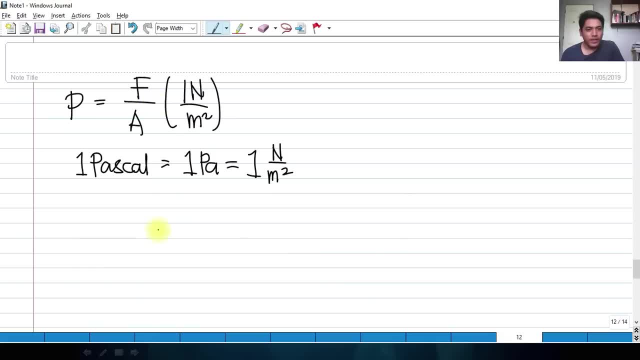 And we say that this force is actually what It's actually: always perpendicular to the surface to which it acts. For example, we have this plate, okay object with an area A. So the force acting should be always perpendicular to the normal or the surface of the object. 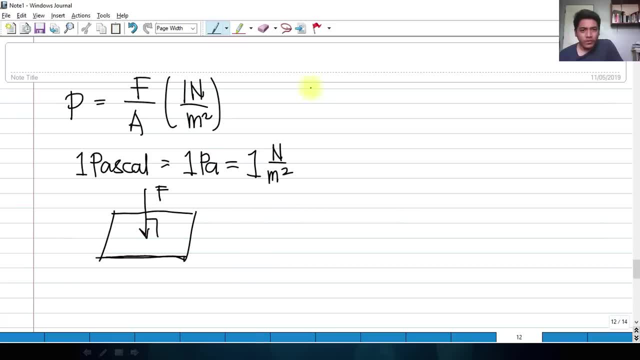 So that is the pressure. So in our equation, if you're going to look at this equation, if we increase the force acting per unit area, well, of course, if we, the pressure here is actually force over area- What if we double the force? 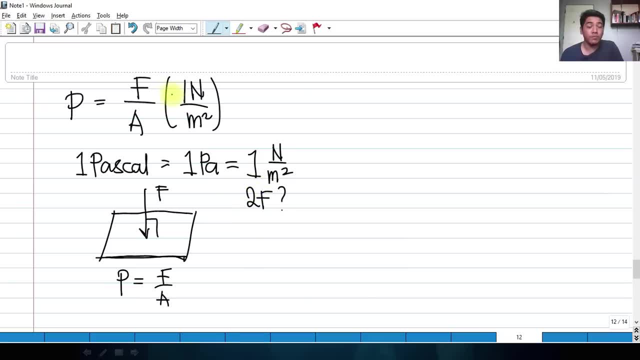 Okay, what will happen is that, since this is since force is directly proportional to the pressure, so we will be having force. pressure is equal to twice the F over. Okay, so our pressure will increase, actually by 2, also because of the increase in the force. 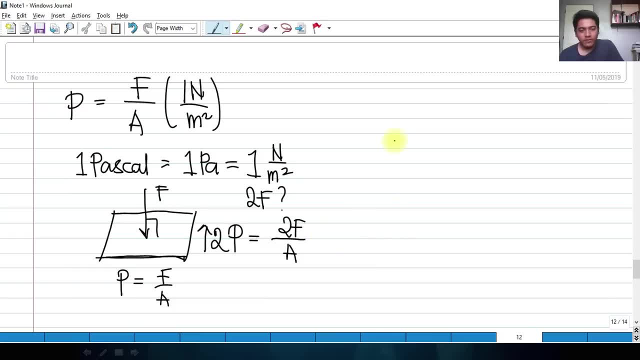 So what will happen if we try to apply a force to a very small area, okay, much smaller than this? So what will happen? let's say we have here an object, okay, and it's acted by a force. This has an area, A prime, which is basically smaller than this. 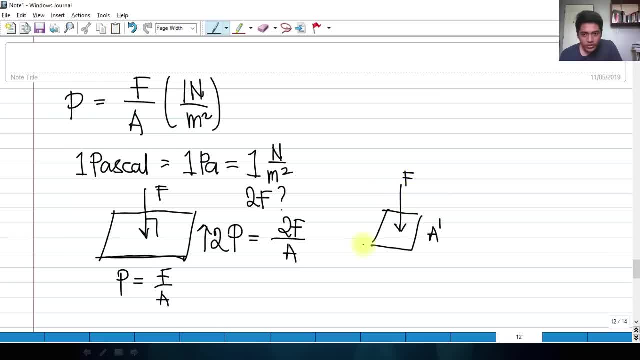 So we have the same Force applied. So the pressure here is actually much greater than the pressure here because the area is now smaller. And we, if we decrease the area to which the force is acting, what will happen to the pressure? 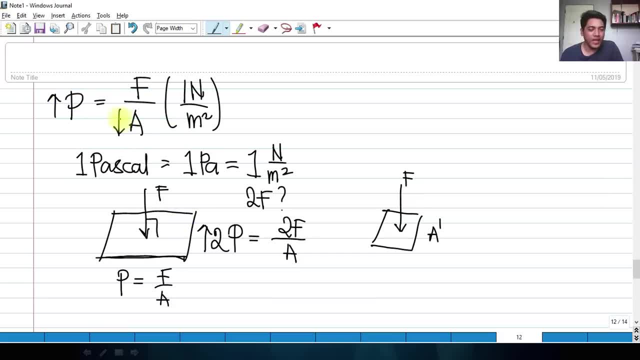 It would increase. Okay, so because this has the area and the pressure as indirectly proportional, or indirectly proportional to each other, or inversely proportional to each other, so that if we're going to decrease the area, the pressure will increase And, of course, increasing the area to which the force is acting upon well will also decrease the pressure. okay, 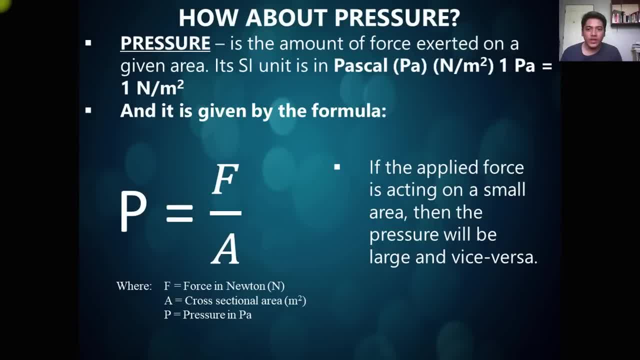 So that's the basic concept of the pressure. So in other words, if the applied force is acting on a small area, then the pressure will be large, and vice versa. okay, So take note that pressure has many units. Its SI unit is only given by Pascal, but we can convert pressure. 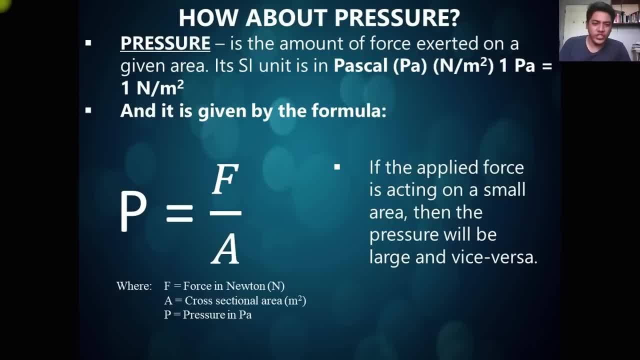 We have different types of units, such as Thor, MMHG, Bar, okay, ATM. We have many units for pressure, But for now we're going to talk about the Pascals. okay, Again, the area here is the cross-sectional area of the object to which the force is acting. 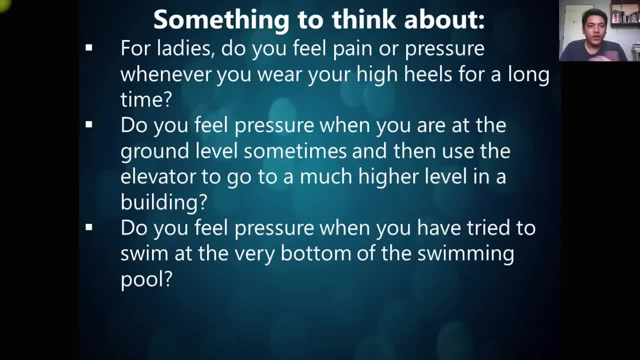 So something to think about when we are dealing with pressure. Poor ladies, do you feel pain or pressure whenever you wear your high heels for a long time? Well, of course some of our friends. you know who's going to party? those ladies are wearing high heels, maybe five inches. 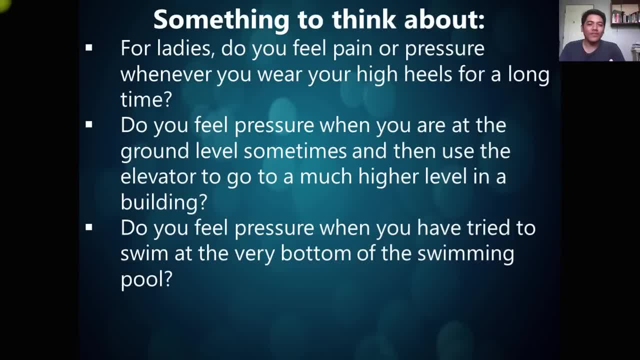 So what happens? the tendency is that whenever they wear that for a very long time, they will feel pain in their feet, okay, Or even in their legs. Why? Because there is the presence of pressure. If you're going to recall from our equation a while ago that the 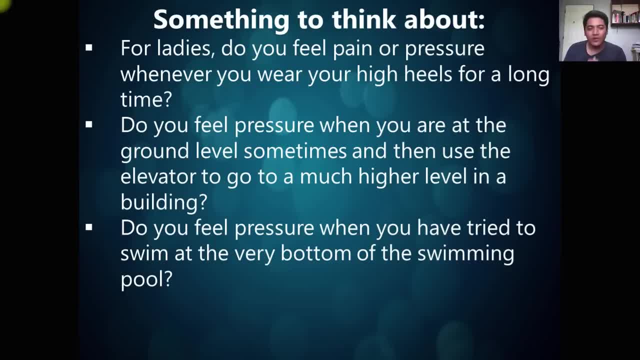 Pressure is inversely proportional to the area- cross-sectional area. So, for example, your friend is wearing a high heels, So the tendency is that the weight now becomes the force, because weight is also a force. So it is now acting on the very small cross-sectional area of the heels. 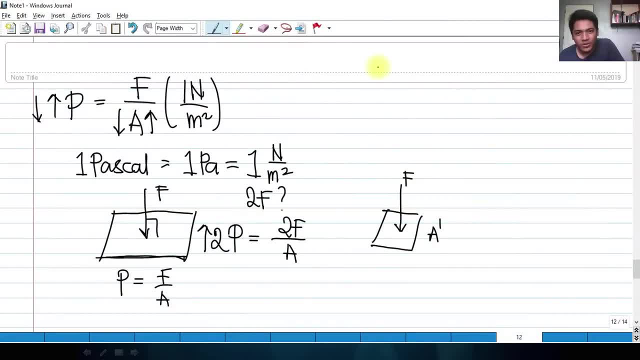 Imagine, of course, if we're going to draw that. So let's just make this as an exaggeration. okay, Suppose this is the heels of your friend and this is the force acting, okay, on this heel of the shoes, of the five-inch shoes of your heels of your friend. 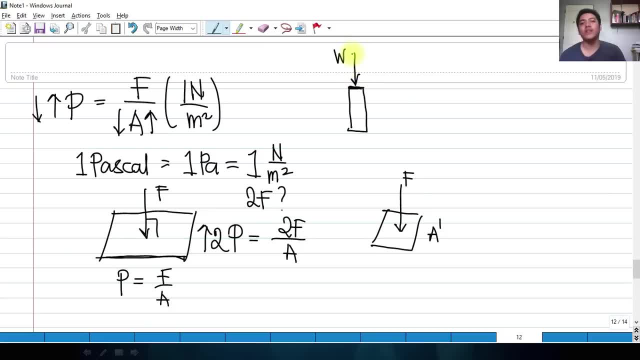 So this force is actually her weight. okay, And let's say that if the weight of the user, of your friend, is really large- in other words, he's a little chubby- what will happen is that the pressure That your feet will feel is very large, because the cross-section here is actually a very small square. okay, 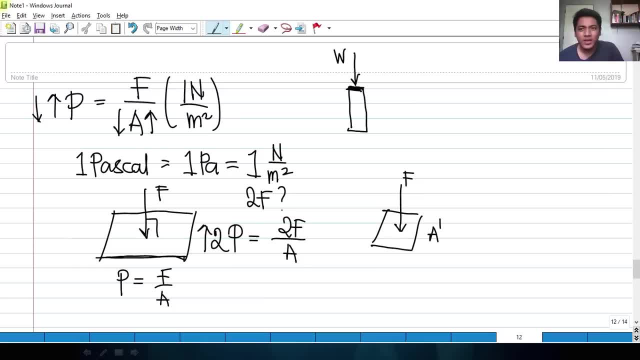 Area of a square, So very small area. So that's why we cannot actually wear- or ladies cannot actually bear wearing that high heels for a very long time, because the area to which their weight Is acting is on a very, very small area. okay. 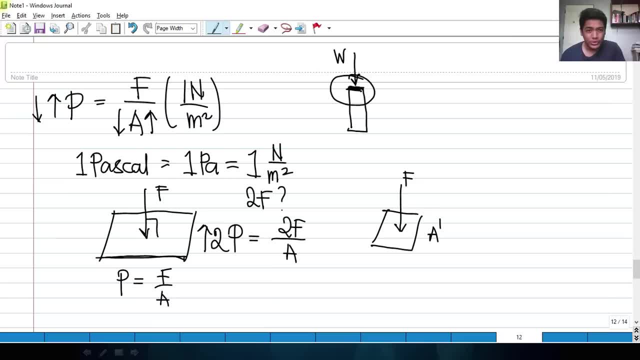 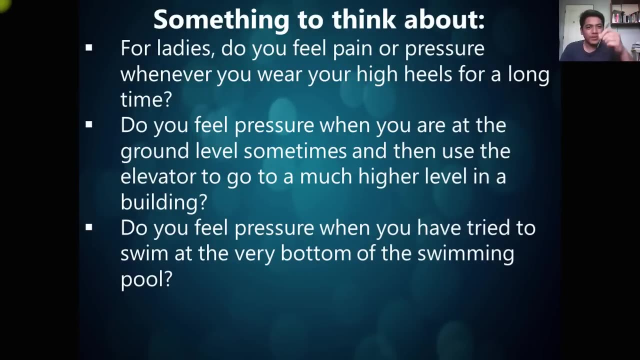 Compared to when we wear shoes okay, The normal shoes, the area of our shoes okay is really really large compared to the area when wearing high heels okay. So the point is that there is a great pressure in the high heels of your friend who is going to wear these high heels okay. 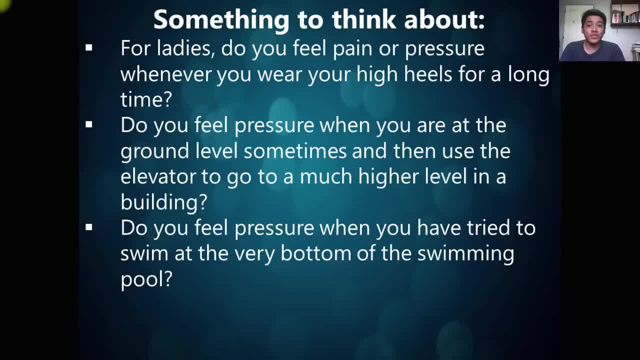 So number two, number two: do you feel pressure when you are at the ground level and sometimes, and then use the elevator to go to a much higher level in a building? okay, so well, of course, sometimes we are at the ground level and we try to ride the elevator, and that from ground to 30th. let's say that is. 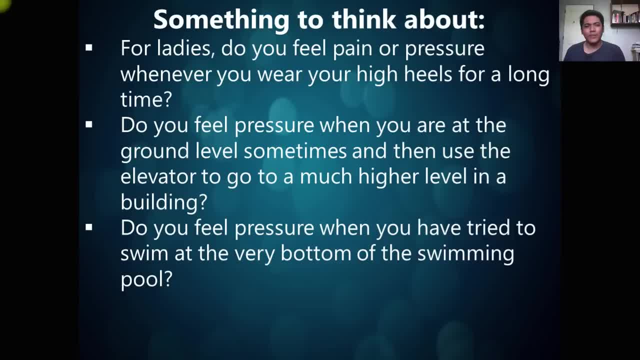 constantly going up. okay, so what happens is that the tendency is we feel pressure in our ears, okay, and sometimes there is a tinkling sound in our ears because of the pressure, okay, so not only because the pressure is limited by this formula, but also the pressure is actually has another. 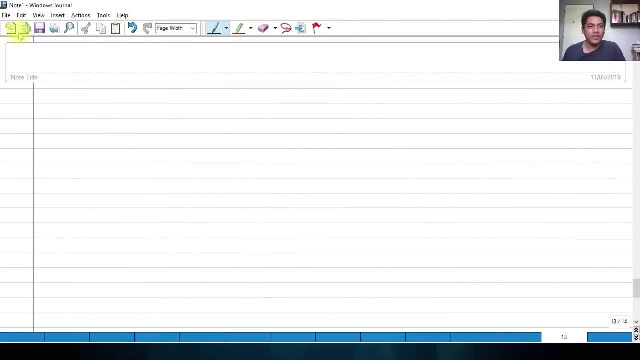 formula of which the pressure to which our body feels is actually equal, also into what we call the raw gh, and it is a function of height. so raw gh is actually the row, is the density, g is the gravitational force. okay, gravitational force, acceleration due to gravity. and this is now the 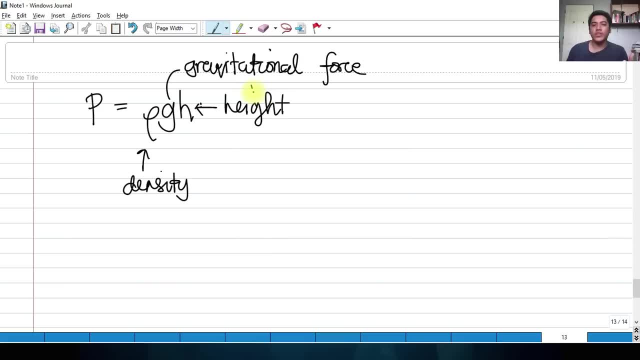 height. so whenever we go to a higher elevation we experience pressure. for example, we ride the flight from manila to daavu. we're we're actually riding a, an airplane, so at very high height now we feel pressure in our ears because pressure is also a function of height. so 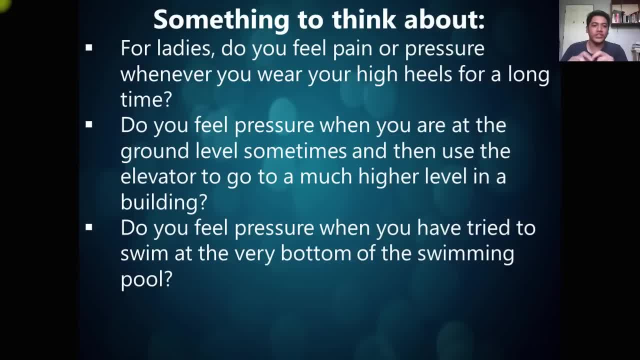 we have this following formula: pressure is also equal to raw gh. so number three: do you feel pressure when you have tried to swim at the very bottom of the swimming pool? well, actually, we always feel that whenever we try to swim at the very bottom of the swimming pool. if you don't, 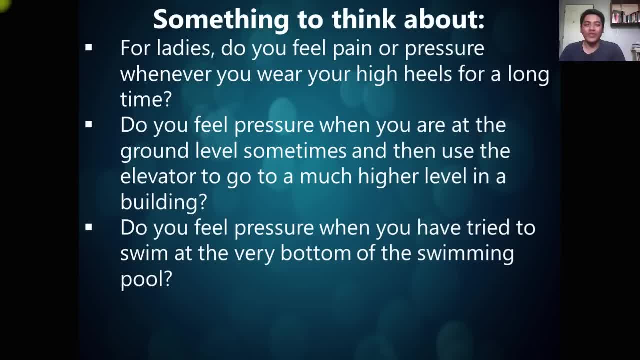 uh know how to swim. good for you, you don't feel any pressure. but but most of us maybe have experienced this- that whenever we go deeper, okay, in the, into the deep of the swimming pool, what happens is that the tendency is we feel pressure in our nose, okay, and maybe in our ears, and then 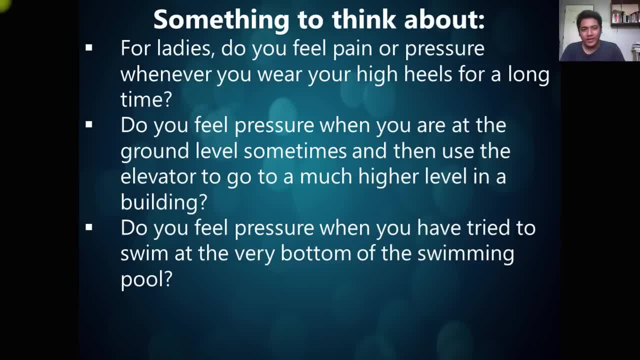 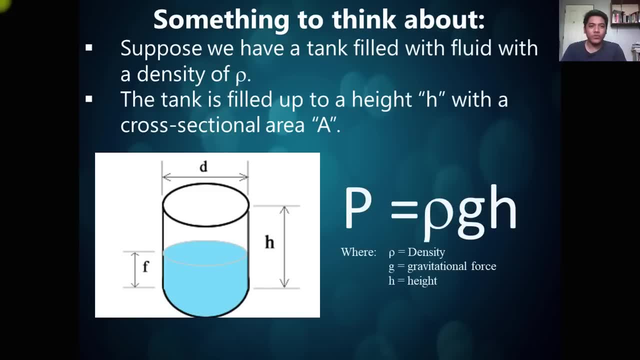 maybe in our head because of the pressure and, uh, that is all, because of the formula raw gh. so suppose we have a swimming pool and we feel pressure in our nose, and then we feel pressure in our ears, and then we have a tank filled with a fluid density rock, just like what i've said. 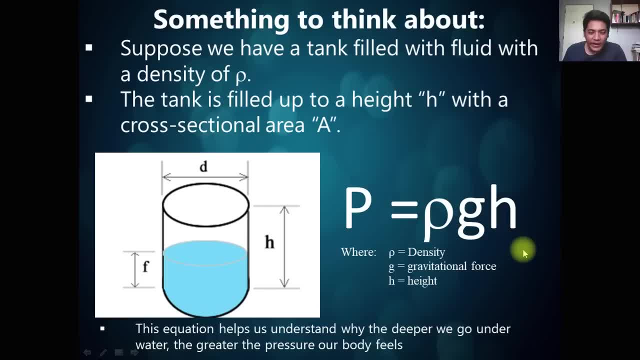 a while ago, that pressure is equal to raw gh. okay, so at the very bottom of this tank, okay, there is a pressure, and that pressure is actually raw gh. okay, not including the what we call the atmospheric pressure. but what? later on we'll be discussing that. so this equation helps us understand why. 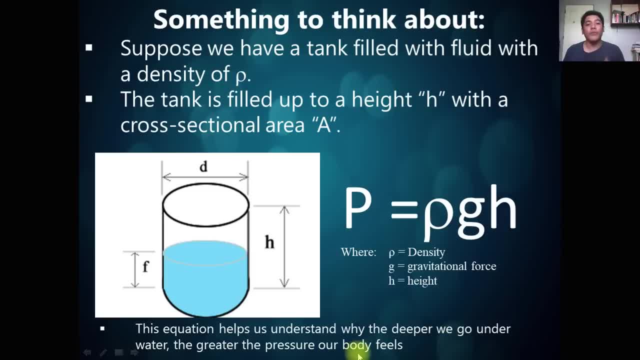 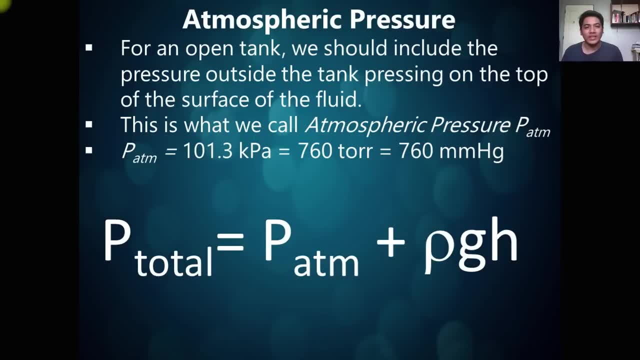 the deeper we go underwater, the greater the pressure our body will have to deal with. okay, so atmospheric pressure. there's also what we call the atmospheric pressure, and that is basically defined as the p sub atm. okay, and when do we use that constant? okay, for atmospheric pressure. well, of course, if we're going to use that for an open tank, we should include the. 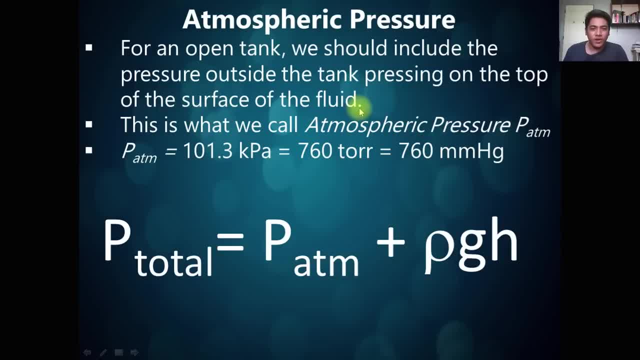 pressure outside the trunk, pressing on the top of the surface of the fluid. in other words, whenever we have an open- okay, an open- tank and it is actually acted by the atmospheric pressure, and if we're going to measure the very pressure at the very bottom of that tank, we should include 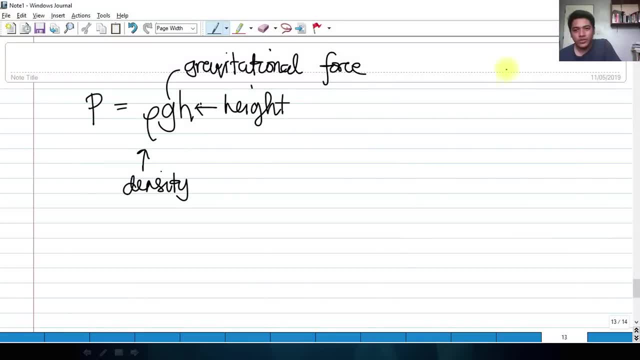 the atmospheric pressure for you to analyze. what i'm trying to say is that whenever we have an open tank and this tank, for example, is actually filled with water, okay, up to this level, to a h if we want to- to measure the pressure at this point, at the very bottom of the of the tank, what? 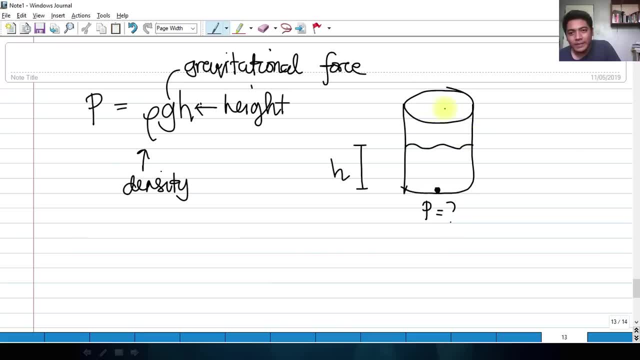 is the pressure there. so there is what we call the atmospheric pressure, and for every open tank we must include that in our computation. so the pressure at the very bottom of this tank is the atmospheric pressure, okay, multiplied by the pressure due to rho gh. so the total pressure at the very bottom for an open tank acted by the 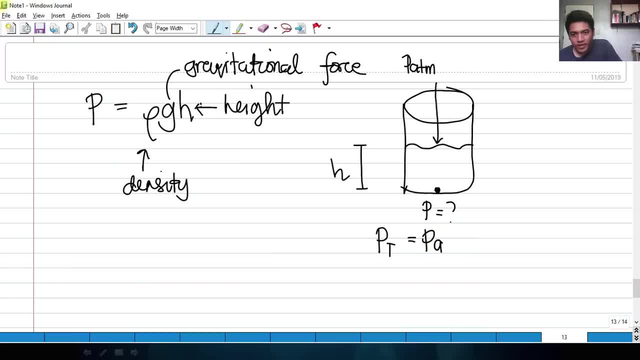 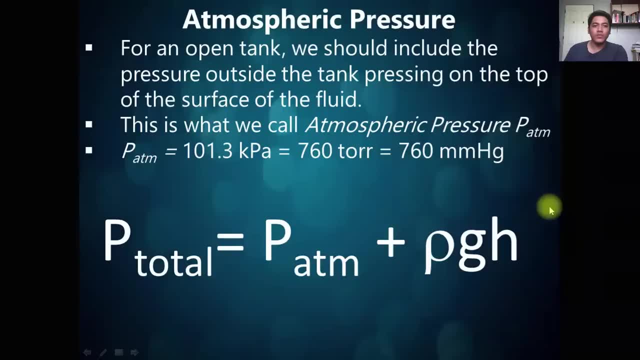 pressure, or the air, is actually the atmospheric pressure plus the what we call the rho gh. okay, so atmospheric pressure is actually equal to 101.3 kilopascals, and that is equivalent to 760 tor, equal to 760 mm hg, and that is basically the atmospheric pressure of the tank. okay, so? 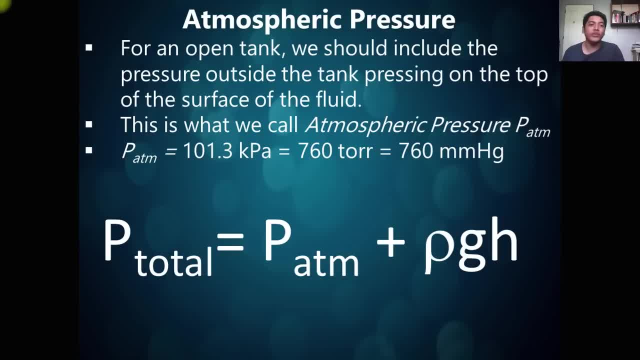 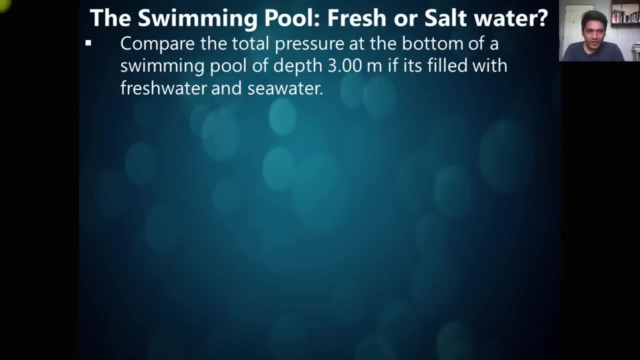 that is basically equal to 1 atm. all of these are units of pressure. okay, so 101.3 kilopascal, or in other words one, one other words one, one point three, two, five kilopascals for accurate uh computations. okay, so for this problem, the swimming pool fresh or salt water? so compare the total pressure at the 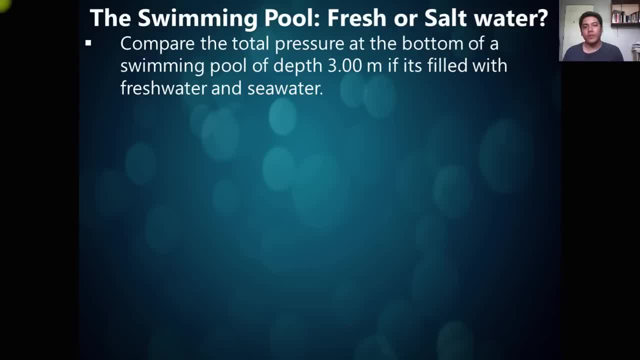 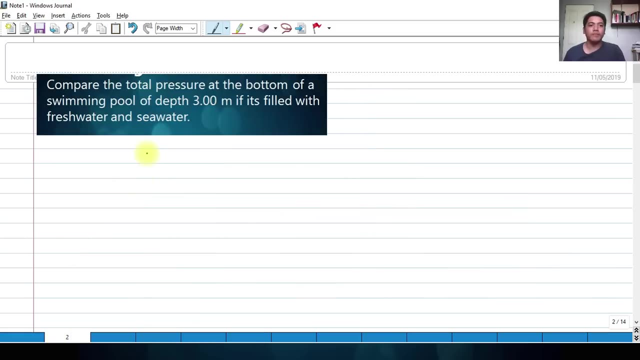 bottom of a swimming pool of a depth three meters, for about nine, nine feet, or eight feet if it is filled with fresh water and seawater. so first we're going to compute the pressure when we are, when we go, we are going to use the uh fresh water. okay, so let's calculate. 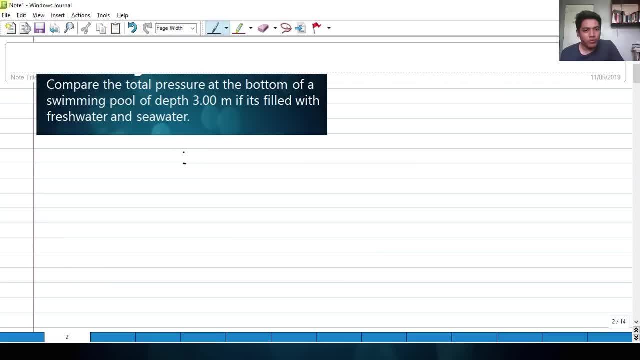 so, for example, here is our pool. okay, here is our pool. okay, this pool is filled with what we call the first and it's high. okay, it's actually three meters. so that is for a three meters height. so we're going to compute now the total pressure at the very. 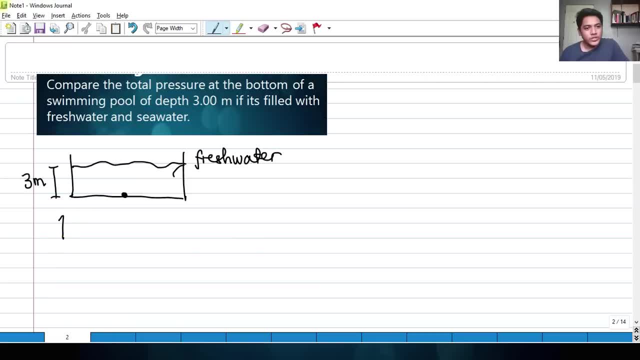 bottom of the spoon. so the total pressure is actually P. total is P atm, because this is an open swimming pool, so we have to include the pressure due to atmospheric pressure. oops, so that is added to the pressure. Rho gh. so we're going to include pressure- atmospheric pressure. this is for num letter a, so one. 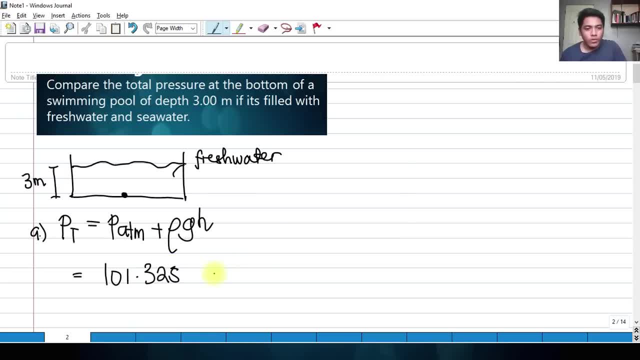 oh, one point three. two, five or one one point three. let's be consistent, right? let's do it again. the pressure, atmospheric pressure, is one oh one point three kilo pascals plus the Rho. what is this? the density of water is one times ten, raised to three kilogram. 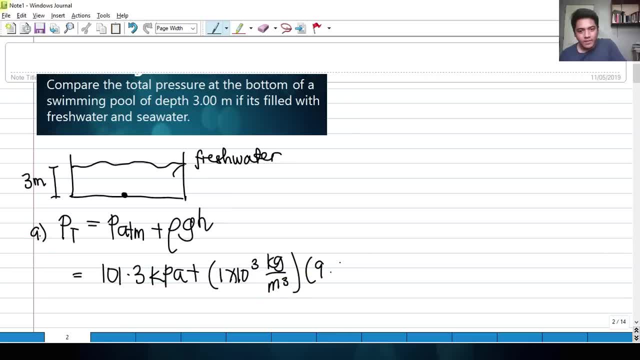 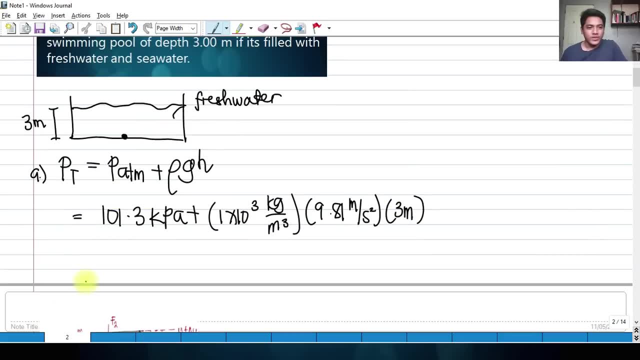 per cubic meter multiplied by nine point eighty. one meter per second squared, and that should be multiplied by three meters. so what are we going to get? here is actually one oh one point three kilo pascals one times 10 to scale to great. okay, let me just compute nine point eight. 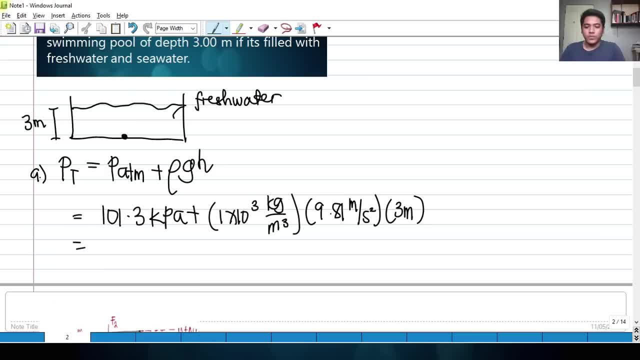 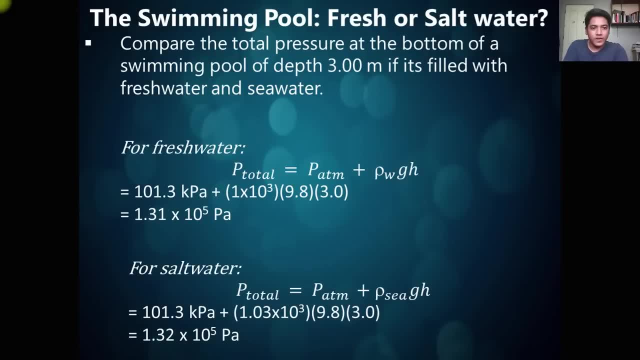 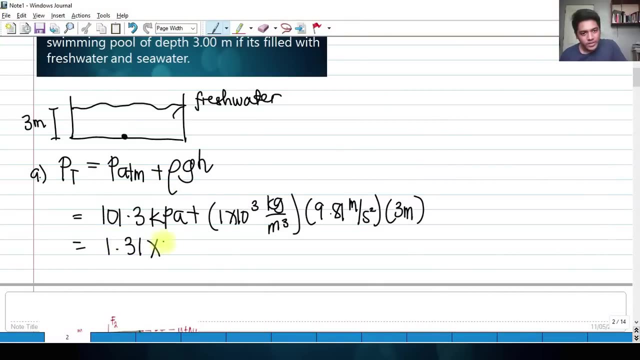 one there three meters, so 130 point seventy three. okay, so let's check I: or one point 31 times 10 raise to five, Farceur, so one point 31 times 10 raised to five, five cos or engineering in engineering mutation, yeah, what might you? 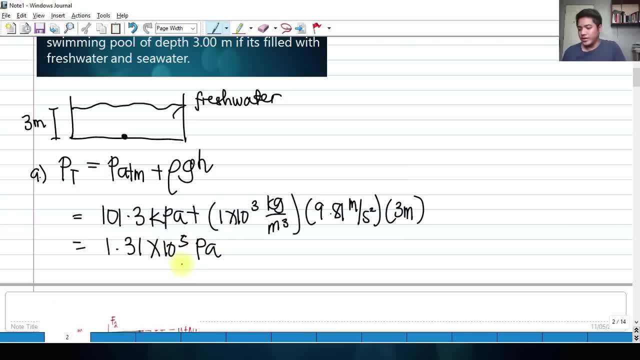 have done here? you know you have collected five. Well, you will just calculate this. what is excellent? Yes, engineering notation 5 can be calculated 130.73, uh, kilo pascals. so what will happen if we're going to replace this fresh water? 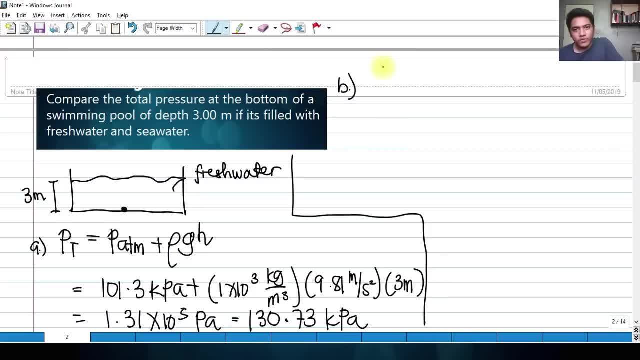 this fresh water by salt water. now for salt water. what will happen is that the same computation we have to include the atmospheric pressure plus the rho of now the sea, or the salt water times, the g times the height. well, of course, the only thing that uh changed here is the density of the uh object. so, from fresh water to sea water. 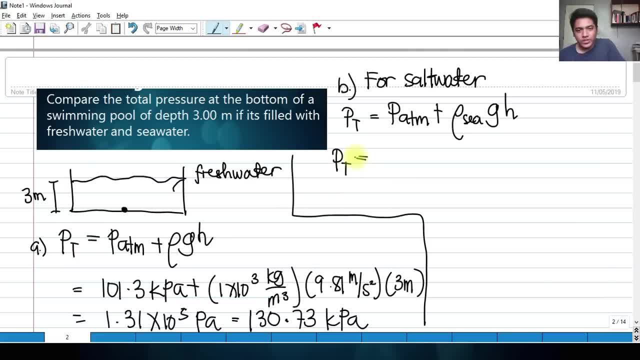 so we have, uh, total pressure is actually equal to 101.3 kilo pascals plus the density of water, of sea water, is one 0.03 times 10, raised to three kilogram per cubic meter, multiplied by g, 9.81 times the height. the 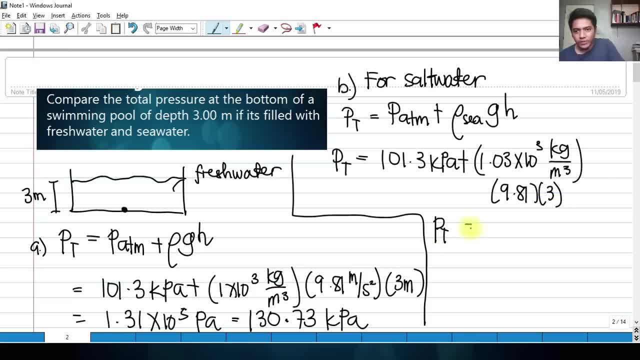 same, that is three. so the total pressure, if we're going to compute for that, is 101.3 kilo pascals plus one time one point zero, three times ten raised to three. nine point eighty one times three. and that is one point. what? one point thirty two. one point thirty two times ten, raised to five pascals. 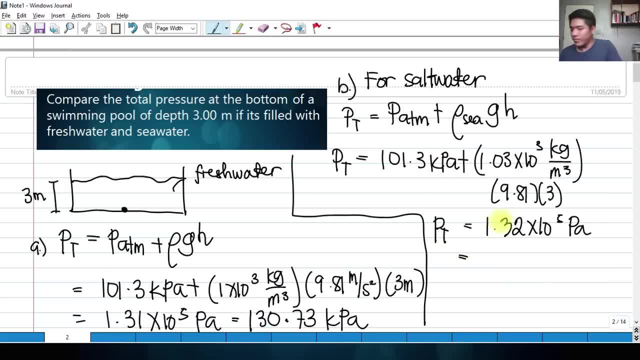 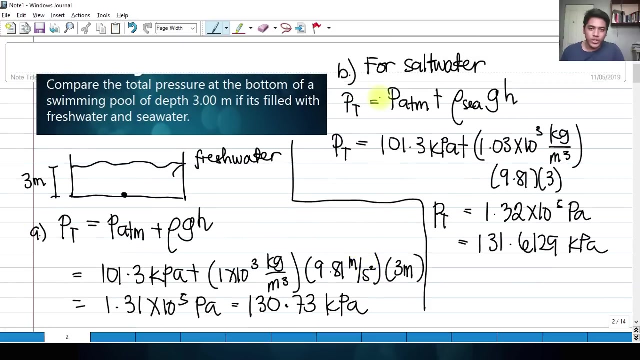 or in in engineering notation, we have one thirty one point one thirty one point six, one, two, nine pascals or kilo pascals, and sorry, kilo pascals. so this is okay. so this is in terms of kilo passes, all right. so there is a big difference in the pressure at the very bottom of the swimming pool. 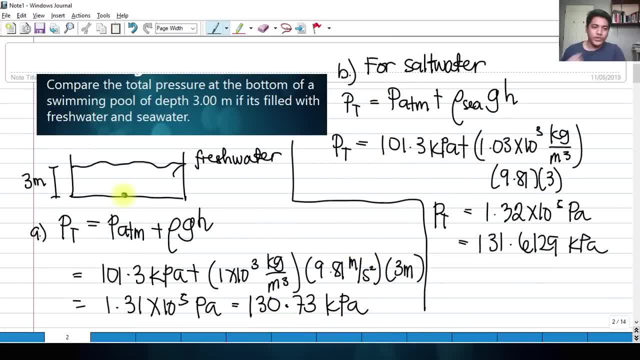 if it is in fresh water. in salt water, as you can see here, the pressure at the very bottom of the swimming pool, if it is fresh water, is given by 1.31 times 10 raised to five pascal, whereas for saltwater that is 1.32 times 10 days to 5 pascal. there is a great difference, so that the determining 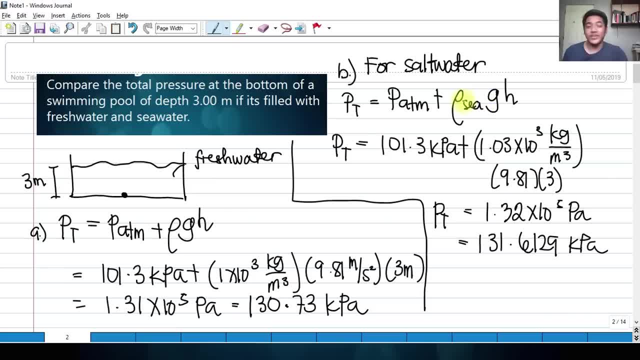 here is actually because of the density, the difference of their density. so that's why we have to include that whenever we swim, we try to swim at the very bottom of a freshwater. the pressure is not really that great. but when you try to swim at the very bottom of a saltwater or seawater, what will happen? 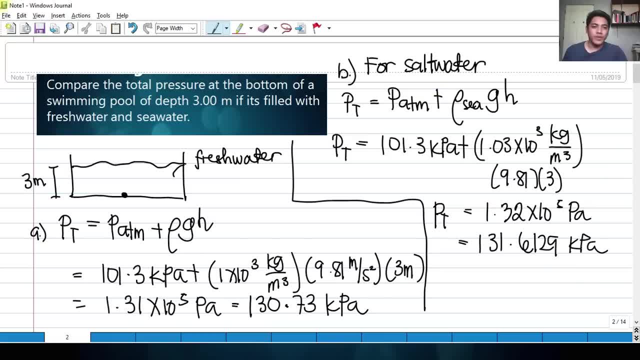 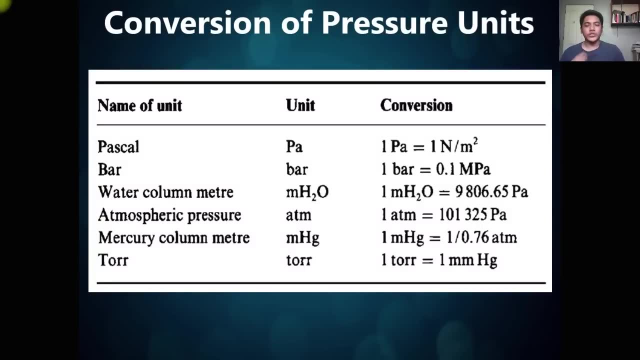 is that the tendency is that you will feel a greater pressure. why? because the density, again, of the seawater is much greater than the density of the fresh water. okay, so let's go back to our discussion. so, conversion of conversion of pressure units: we have different conversion of pressure units. 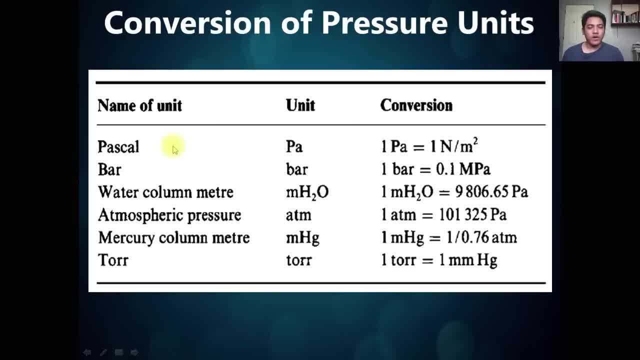 because we have many units of pressure. so Pascal denoted by PA, 1 PA is equal to 1 Newton per square meter and we have what we call the bar. bar is a unit of pressure, or so, in one, bar is equal to 0.1 mega pascals. that is a huge amount of. 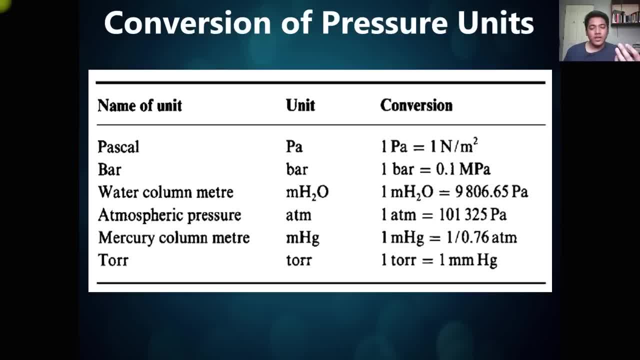 pressure. so 0.1 mega pascals is actually equal to 0.1 times 10 raised to 6 pascals. we have the water column meter. okay, that is the equivalent conversion units. honestly, I don't know that. okay for the, I really haven't encountered. 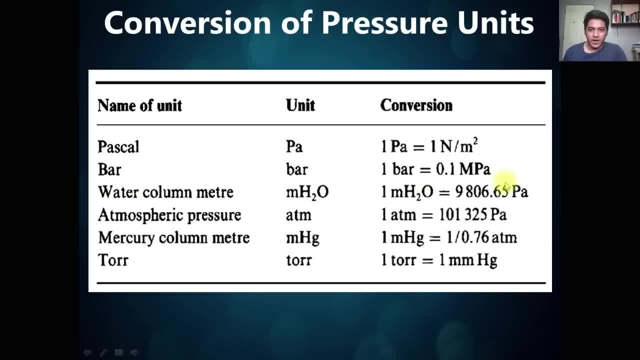 that during my time in my college, but I hope someday you will remember that in your major subjects. so we have the atmospheric pressure: 180 M ATM. 180 is basically equal to this. the pressure- atmospheric pressure is 30 11325 pascare, or what we haveup to record a while ago. 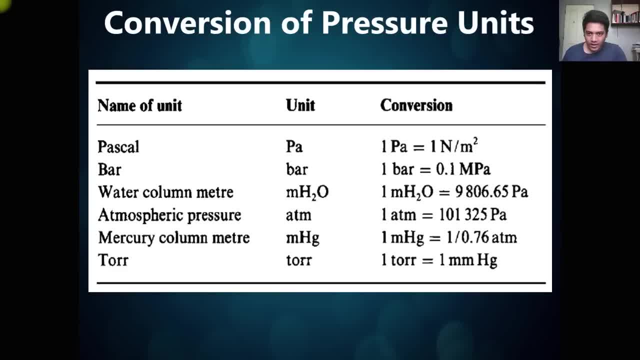 that is 101.3 sins, then the to that 11.3 kilo has coached that location is that is 101.3. 1, march 13th to 10 base to 11.3 kilo radiators across sails, theOMAN. 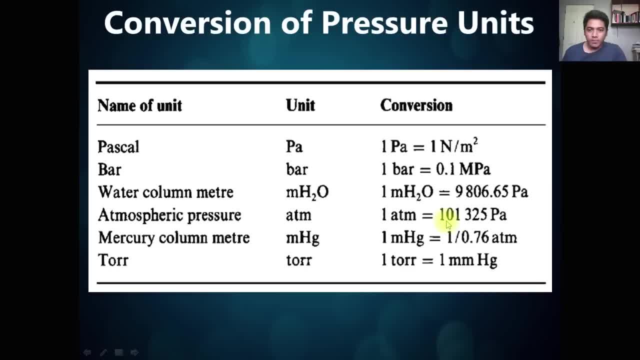 bugs, that is 101.3 than the Rockwell. so the most up, more accurate is one the ground, 0.325 kilopascals or 101.325 pascals. so we have the mercury kilometer given by this conversion and we have the 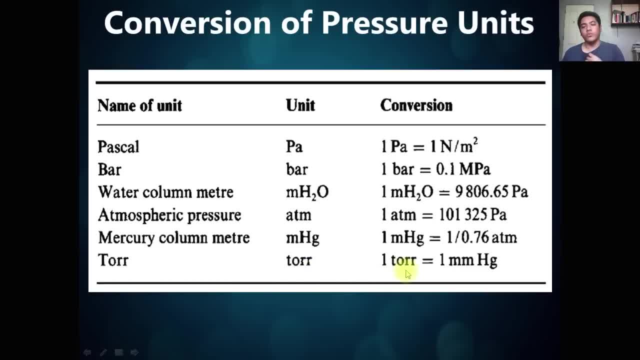 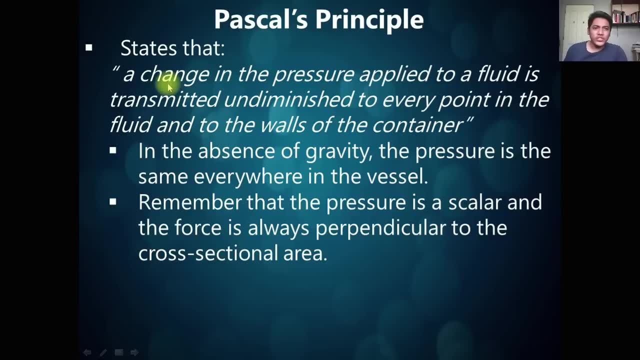 torr. torr is the unit of pressure and one torr is equal to one millimeter hg of pressure. okay, that's basic, the basic conversion of pressure units. so let's go on to pascal's principle. so pascal principle states that a change in the pressure applied to a 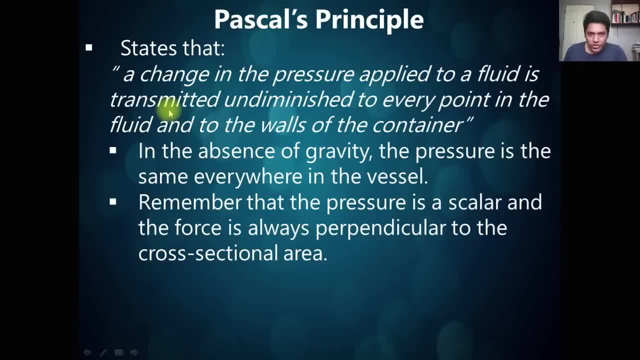 fluid is transmitted undiminished to every point in the fluid and to the walls of the container. in other words, pascal's principle: whenever we have a fluid inside and we apply force, that results to a pressure on the left side, the pressure on the left side must be always equal to the 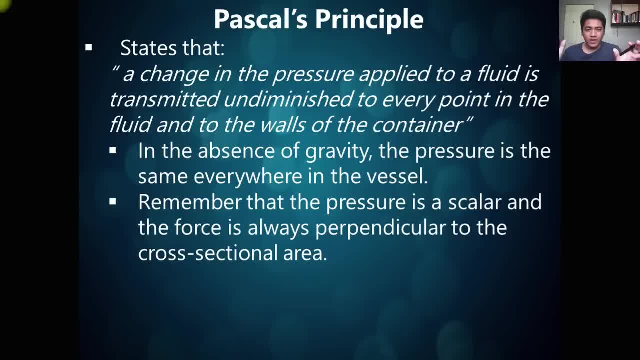 pressure on the right side of the container. okay, the pressure is transmitted undiminished to every point in the fluid. so, in the absence of the gravity, the pressure is the same everywhere in the vessel. so remember, the pressure is a scalar quantity, but the force is actually a vector. so, but the pressure is scalar, even though. 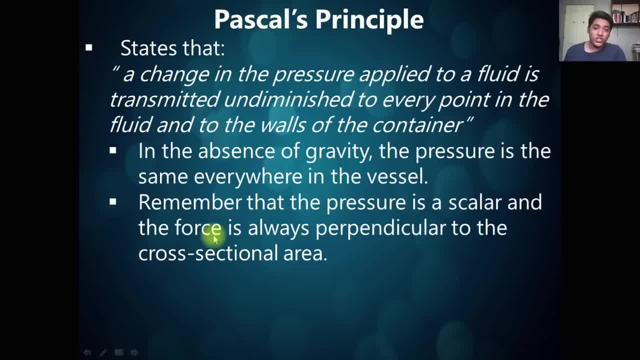 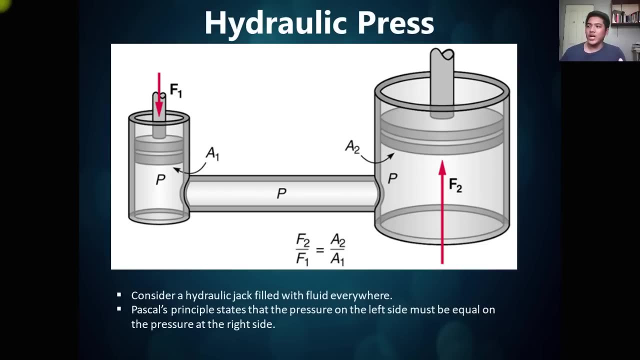 the force is vector and the force is always perpendicular to the cross sectional area. so what will happen here is that, if we have, for example, one application of pascal's principle is actually what we call the hydraulic jack, this hydraulic or hydraulic press or hydraulic jack, this hydraulic press is actually. 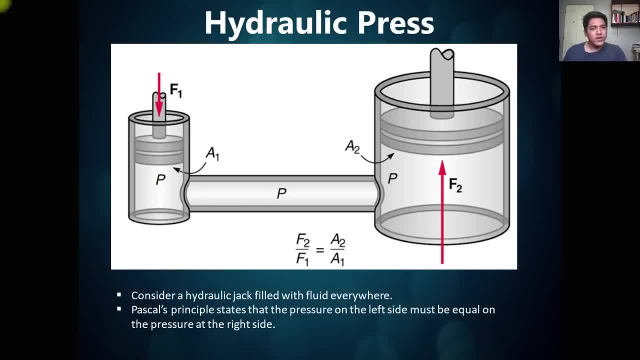 used to lift cars in a carlifting service station or in a company where cars are being manufactured. okay, so consider hydraulic press or hydraulic jack. this hydraulic jack is filled with fluid inside. so pascal's principle states that the pressure on the left side, this left side. 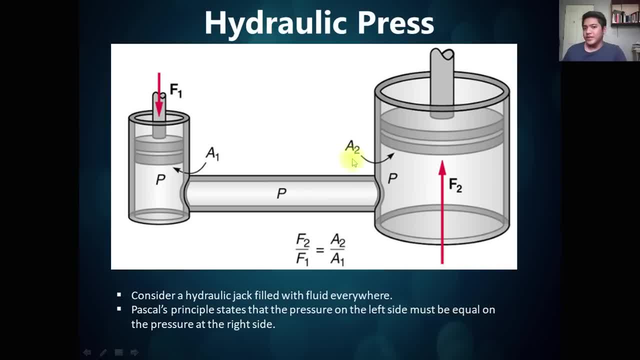 must be equal to the pressure on the right side. so well, of course, for example, if we have this hydraulic press, okay, if we apply force here on the left side, okay, for this cross-sectional area a1, we are actually producing the pressure because this force is acting perpendicular to the 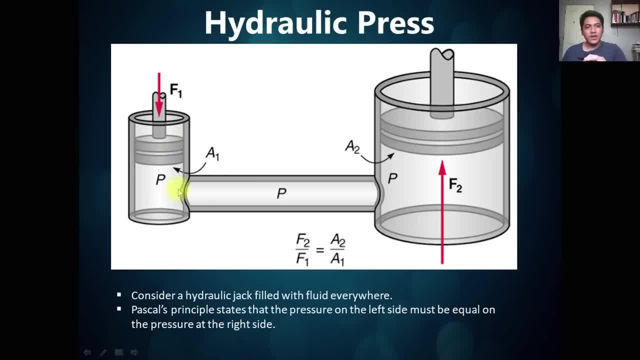 cross-sectional area a1 and according to pascal, if we create pressure here, the pressure we created here must be also equal to the pressure that is produced here. so actually, if we're going to apply force here, fluid will be displaced so that there will be a force upward- f sub 2- that is acting on. 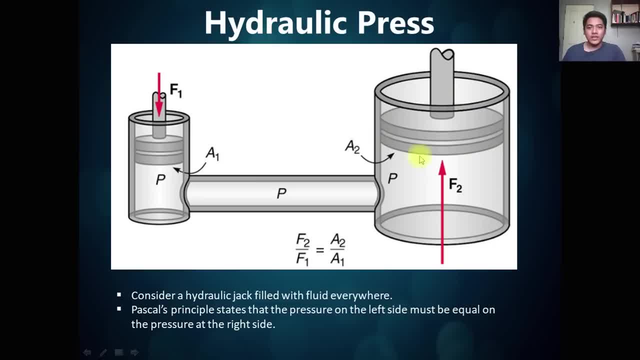 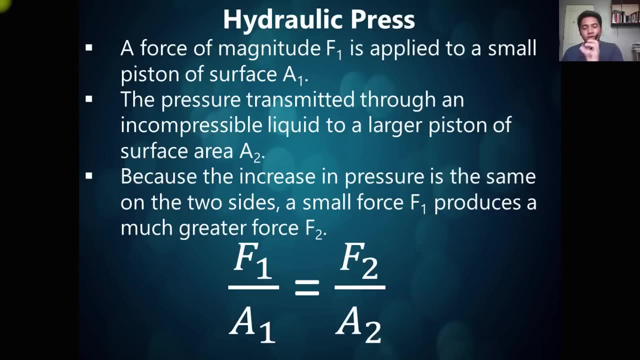 the much bigger cross-sectional area of this hydraulic press, a sub 2 so, but the pressure remains the same according to pascal's. okay, so what are we i'm trying to say is that, because of the equal pressure on the left side and on the right side, we have this following formula: okay, so f1 is. 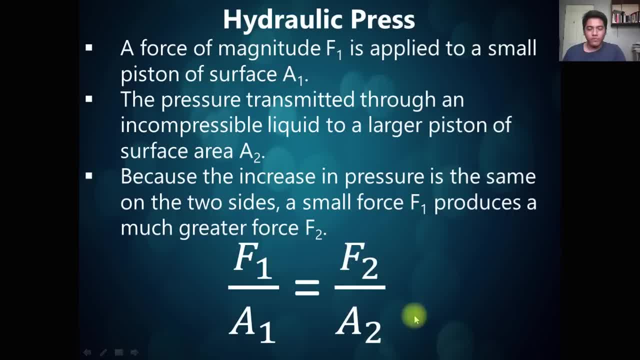 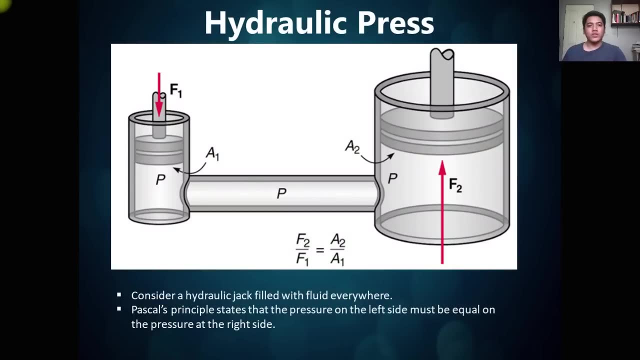 equals to a1, that is pressure 1. that is equal to f2 over a2 because the pressures are equal. so because the increase in pressure is the same on the two sides, a small force on f1 produces a much greater force, f2. so, uh, let me just go back to our image. okay, so let us assume that the smaller area 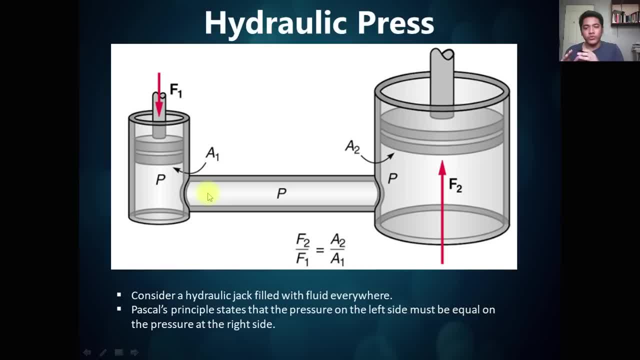 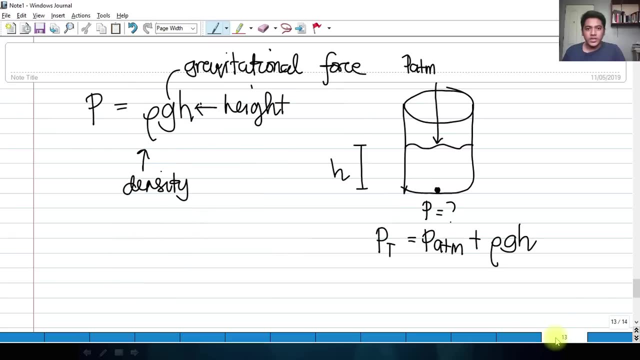 a1 and the smaller force we call that f1, and the bigger area we produce, or the bigger force we produce, is f2 and the bigger area side of the hydraulic press is what we call the a2. so let's just try to compute, okay? so for us to really see the uh beauty of pascal's principle. so we have. 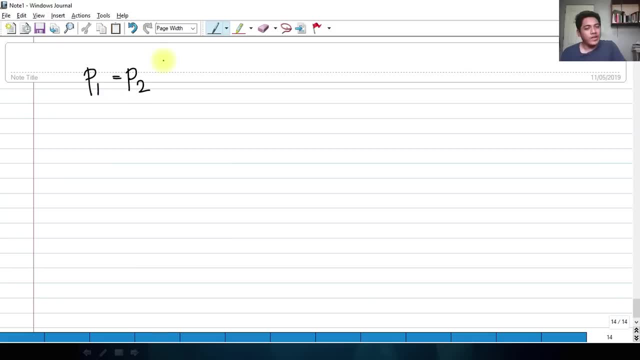 let's say that p1 is equals to p2 according to pascal principle, and if we're going to elaborate on this- f1 over a1, that is, equal to f2 over a2- suppose we want to find the f1. this f1 is the force. 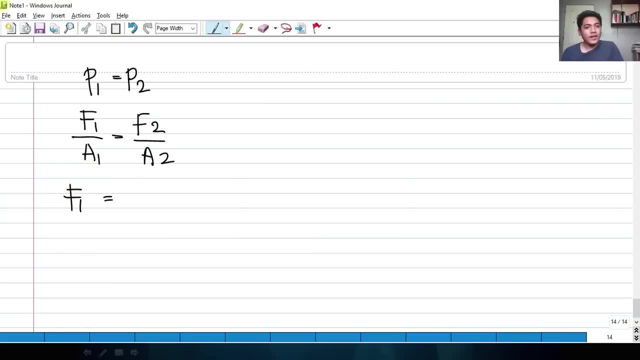 that we are going to apply on the left side. okay, to carry or to lift up a car with a higher uh area, a sub two. so let's go, let's, let's say we, we need to isolate f1, so we have a1 divided by a2. 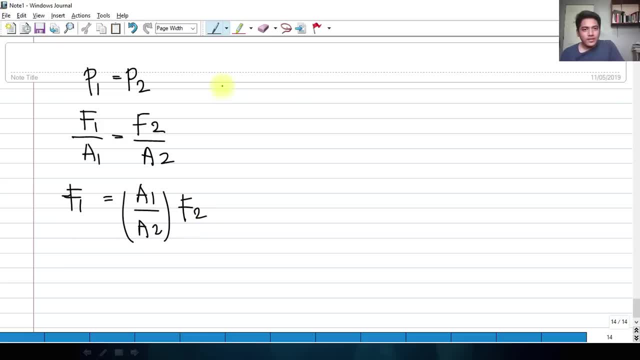 okay, and let's say class that the area of one or the smaller piston, or on the left side of the hydraulic press is equal. let's say to uh, what do we call this? let's say 100 meter square, and well, of course, a2, let's say one meters square meter. okay. 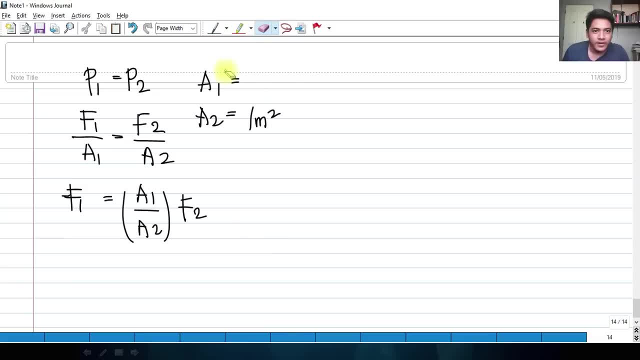 okay, so, ah, let me just make this clear so that, uh, what are we trying to get here? is f2 instead of f1, i'm so sorry. so we have to get f2, because f2 is where we have to leave the car. that is, the right side where we have to leave the car. so when we get f2, f2 or the force onto. 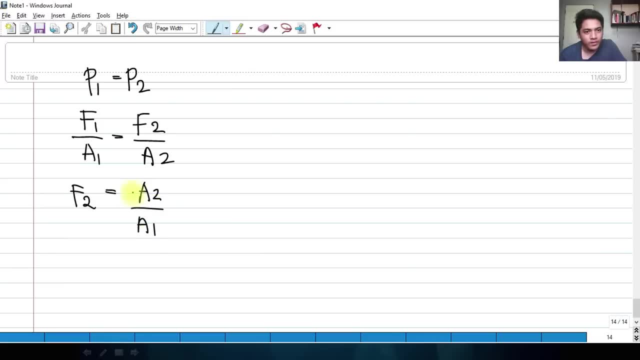 the car, the force is going to be what a2 over a1 multiplied by the force one. let's say that a2, or the area to which the car is being it's to be lifted up. let's say that the area of that is, let's say, 100 square meters. okay, let's just exaggerate this. okay, so, and the area of one to 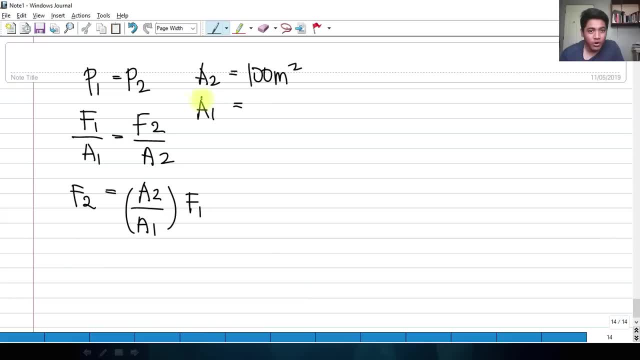 which we are going to uh, apply the force. okay, this area is the smaller area on the left side of our, Let's say, that is 1 square meter. okay, And what are we going to do is to apply 1 newton of force on the left side of the hydraulic press. 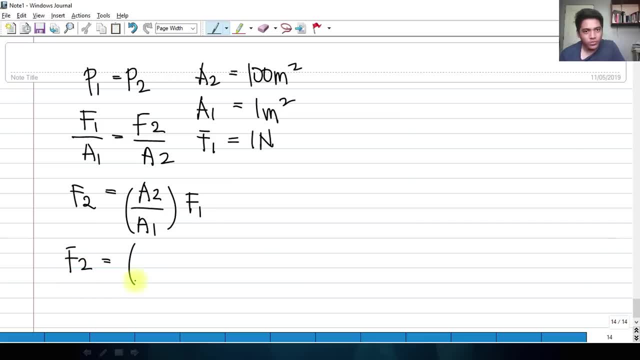 So if we're going to compute for the force 2, we have A2, the area 2 is 100 meters square over 1 meter square, then multiply that by 1 newton. okay, Let's say 1 newton. 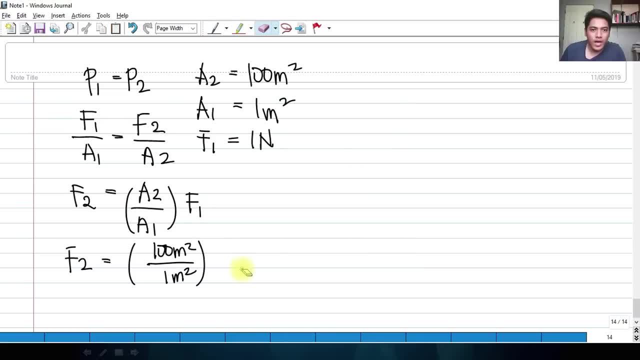 1 newton. what will happen is that, upon evaluating the F2, what will happen is that this would cancel and we are left with 100 times 1 newton, so that we are able to produce 100 newton only by applying 1 newton. 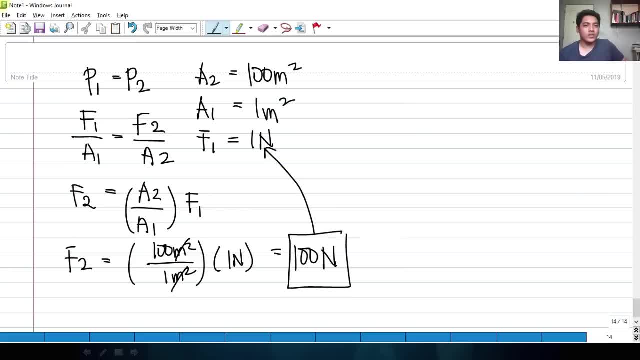 So no wonder why this hydraulic jack would actually perform the lifting of the horse, because small force that we are going to apply on the left side of the hydraulic press would create a greater force on the right side because of the equality in pressure. okay, 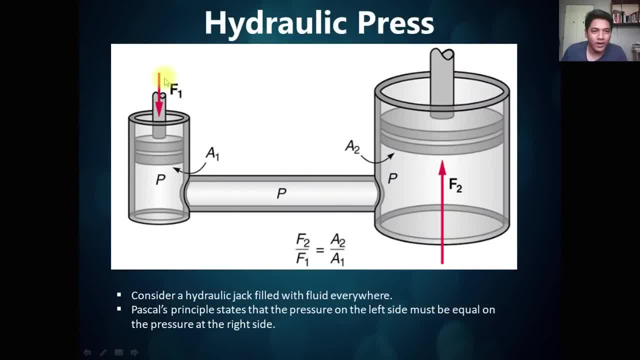 So what I'm trying to say is- this is our first one- 1 newton. a while ago acted by a small area of 1, that is our 1 square meter. then the force that will be produced on the other side or the right side of the hydraulic press would be 100 newton. 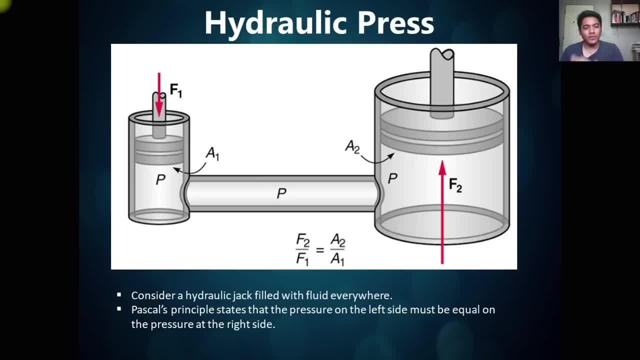 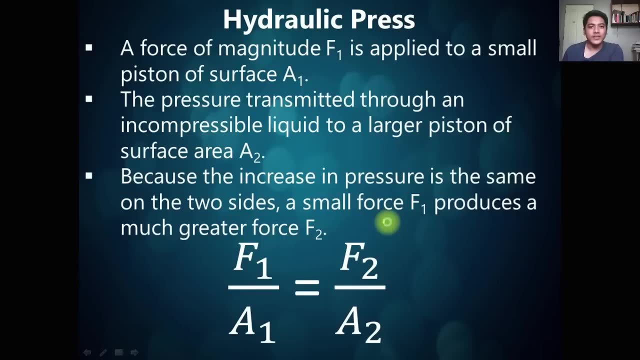 Imagine, From 1 newton to 100 newton. with perfect design or with a good design of the diameter or the area of this hydraulic presses, we can actually lift up cars in a very easy way, okay, So of course, the same amount of fluid leaves on the left and enters on the right side. 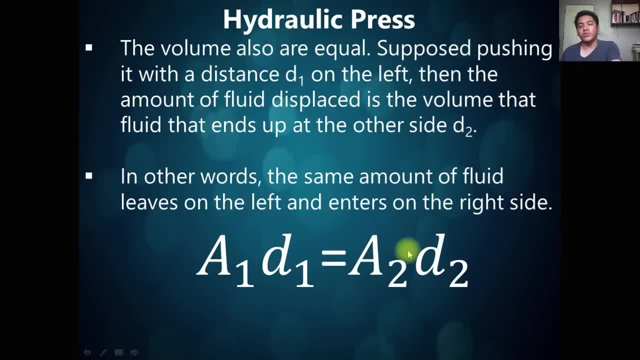 This is actually the volume. A1 times the displacement 1 is equal to A1D2.. So no volume of, So no volume of fluid is left, okay, Or is actually- What do you call this Lost, A force of magnitude 1,? well, of course, we have seen this a while ago, oops. 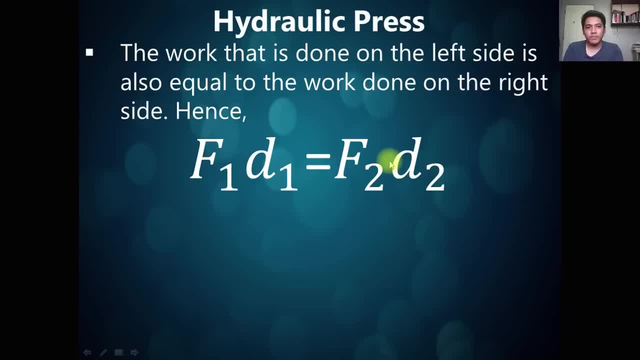 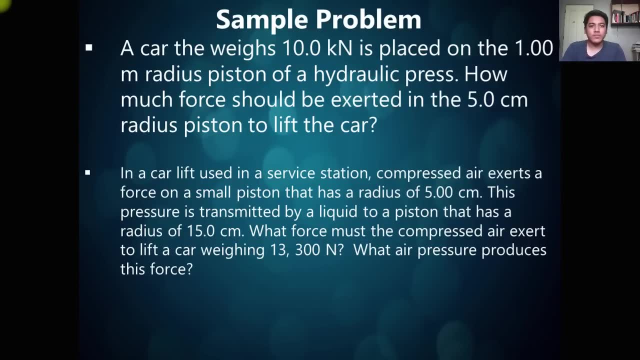 So well, of course, the work done on the left side of the hydraulic press is also equal to the work done on the right side of the hydraulic press, So let's try to have some sample problems. okay, So we have a car that weighs. 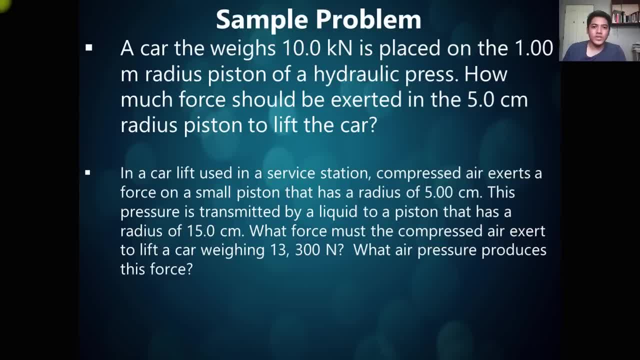 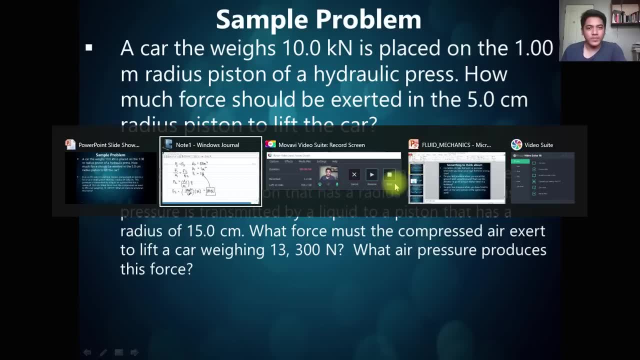 10 kilonewton is placed on the 1 meter radius piston of hydraulic press, How much force should be exerted in the 5 cm radius piston to lift the car? Let me just see if I have copy-pasted it here. 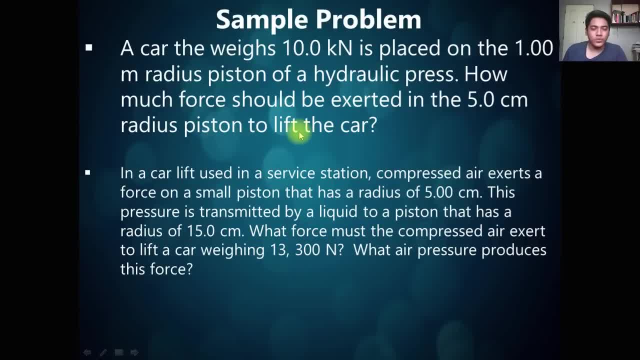 Okay, So I haven't copy-pasted it here. So we have to answer this. A car that weighs 10 kilonewton is placed on the 1 meter radius. Well, actually in In In solving hydraulic presses problems. so we must consider the Pascal's principle: P1 is equal to P2.. 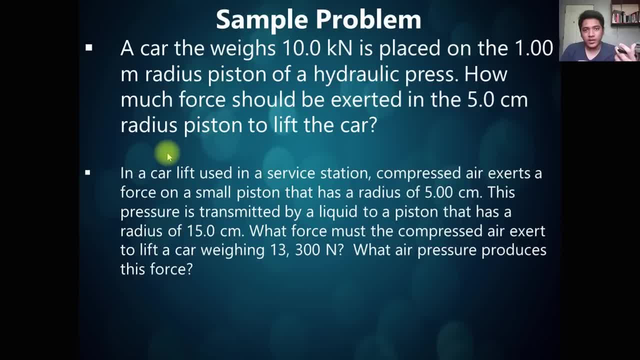 And we must always look for the smaller radius. okay, If we find the smaller radius, which will, in this case, 1 meter and 5 cm, the smaller radius is 5 cm, So 5 cm should be our R1.. 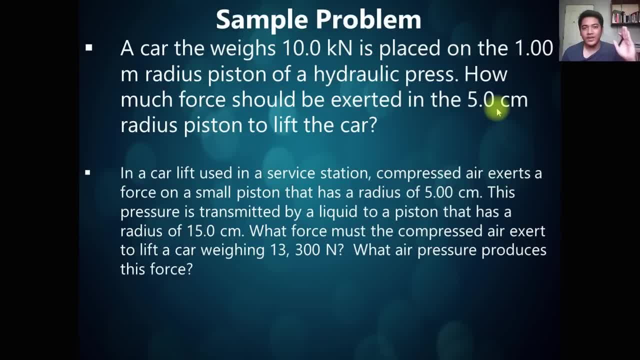 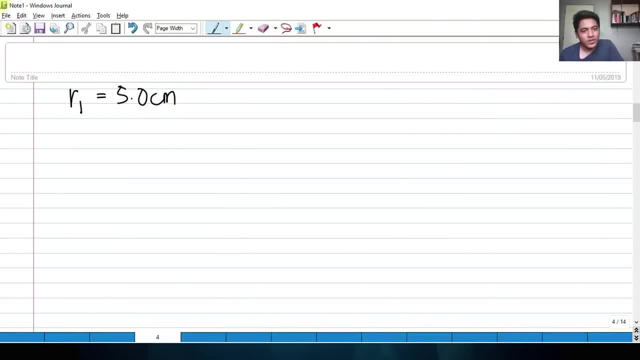 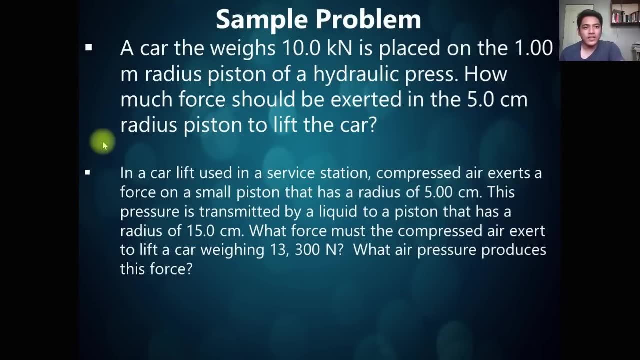 Okay, That should be the left side, Okay. So what I'm trying to say is that we have R1 is given by 5 cm. The problem is asking is how much force should be exerted in the 5 cm. So if that is the R1, this should be the force 1 to which the force is being applied. 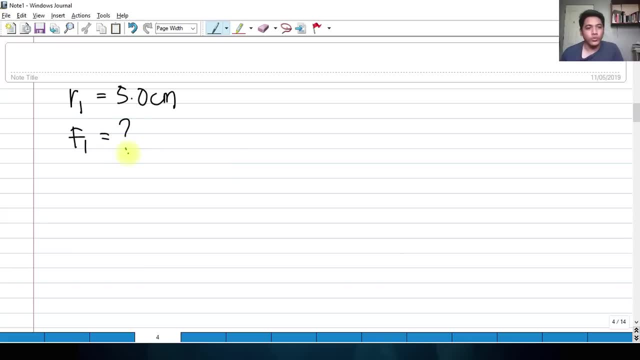 Okay, In order to lift the car on the other side. So that's the unknown, the F1., And we have here 10 kilonewton. By the way, 10 kilonewtons is also a force, That is the F2,, 10 kilonewtons. 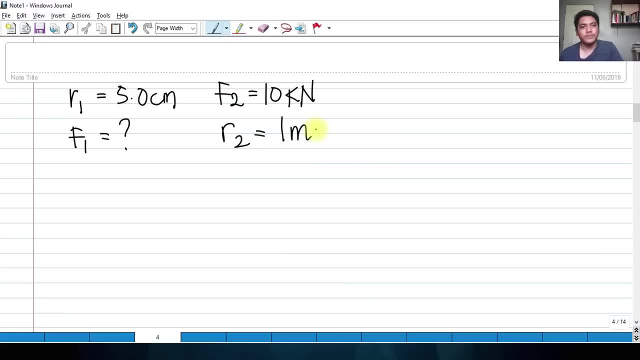 And our R2 is actually 1 meter. Okay, So, applying Pascal's principle, we have: P1 is equal to P2.. That is, F1 over A1 is equal to F2 over A2.. And we are asked to find for the F1. 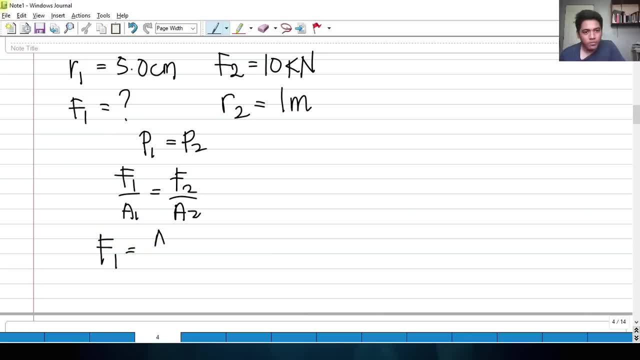 So F1 will now be equal to A1 over A2.. Multiplied by the F2.. So we have now the area. We have to be really careful in this. We are given the radius, not the area, But to get the area, we are asked to find the cross-sectional area. 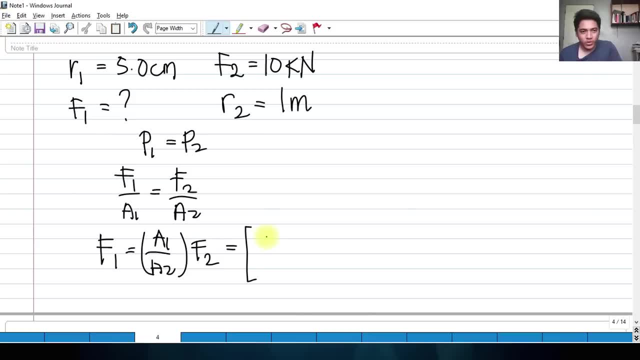 So the cross-sectional area is actually a circle. Okay, So we have pi. We have to convert this 5 cm into meters, So that we have 0.05 meters squared over pi Multiplied by area of 2. That is 1 meter squared. 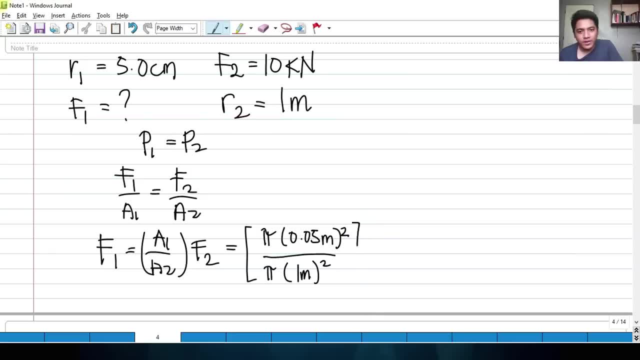 We have no problem with that, And that is basically multiplied by the weight of the car, Okay, So what are we going to do here is simply, as we can see, pi's will cancel, Okay, And multiply that by 2.. 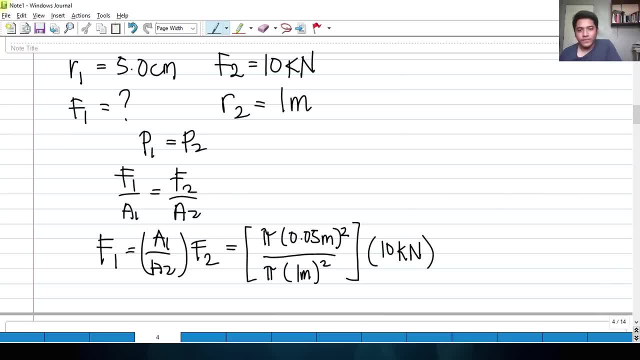 And multiply that by 10 kN, So we have the answer: 25 N. So it's very amazing Why? Because we can lift the car on the right side of the hydraulic press by just simply applying 25 N on the left side of the hydraulic press. 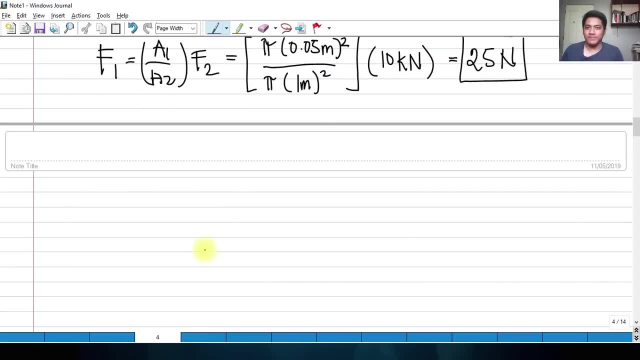 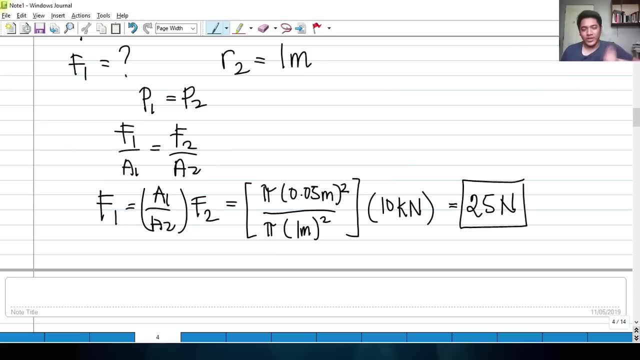 How cool is that? Right So even you, you can actually lift the car. So the best example of that is that the mechanics we can see here. we can see them trying to lift the car by what we call the hydraulic press. 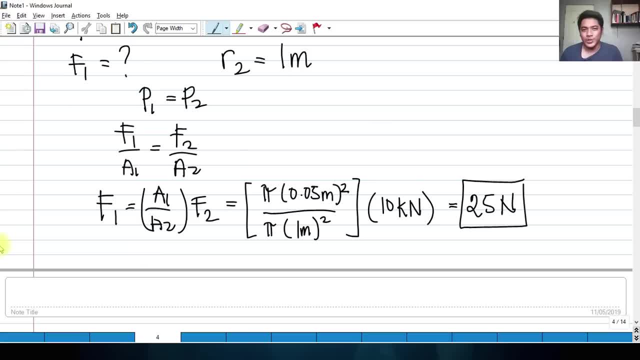 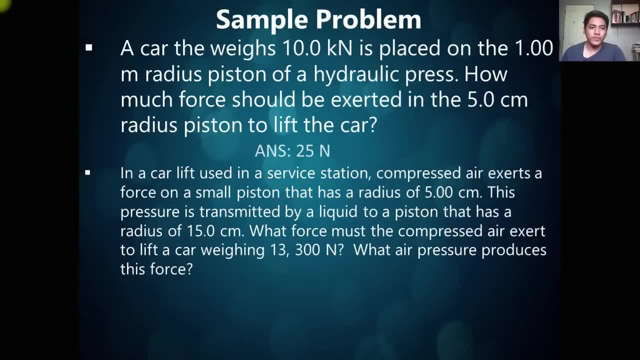 Okay, By continuously applying force so that they are able to lift the car. Okay, That's one basic application of the hydraulic press Number 2.. Or problem number 2. In a car lift used in a service station, compressed air exerts a force on a small piston that has a radius of 5 cm. 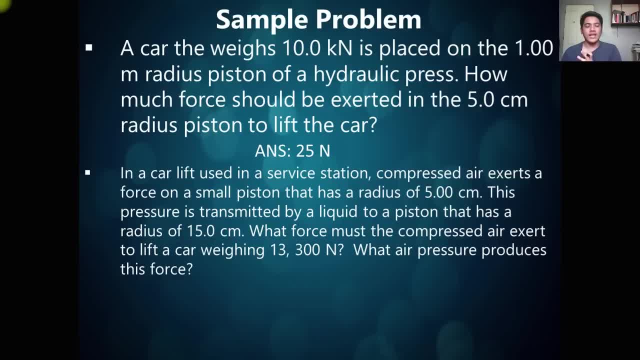 This pressure is transmitted to the hydraulic press. This pressure is transmitted by a liquid to a piston that has a radius of 15 cm. So we have two radiuses again, And 5 cm is the R1, because it's smaller. R2 is the 15 cm. 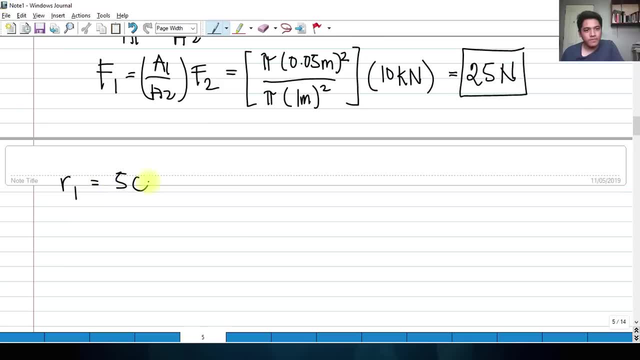 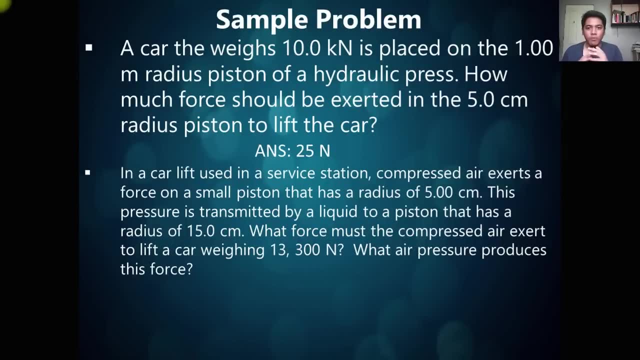 So what are we going to do is to write: the given R1 is 5 cm, R2 is 15 cm. Okay, So what force must the compressed air exert to lift a car weighing 13,300 N? So that 13,300 N, well, of course, is on the right side. 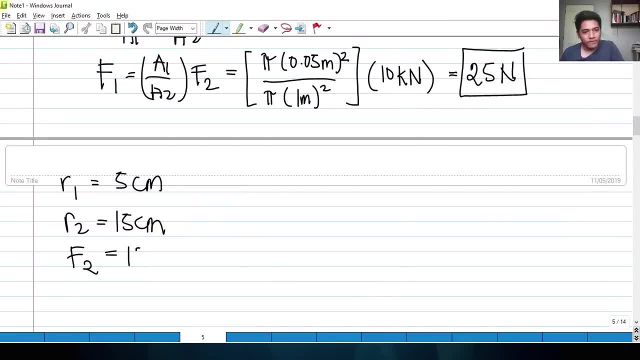 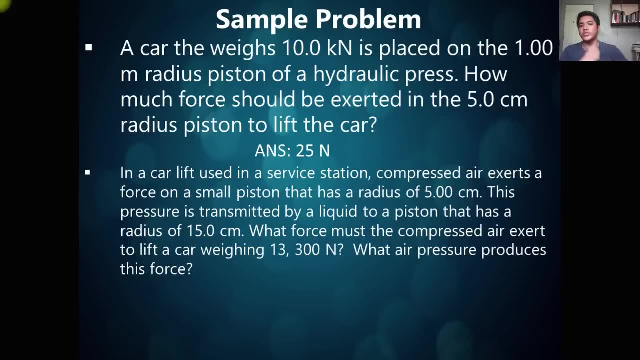 And that should be the weight of the car. That should be F2.. Okay, 13,300 N. What air pressure produces this force? So we have two questions here. What force should be exerted on the left side of the hydraulic press in order for this 13,300 N of car to be lifted up? 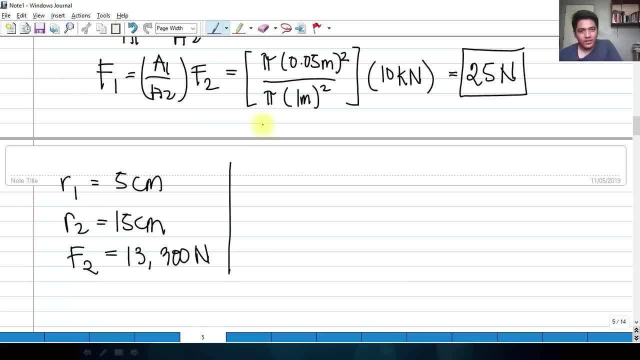 That is again F1. And we have derived again the F1. By the formula: F1 is equal to A1 over A2 multiplied by F2. So we have now A1.. Okay, The area of 1. Cross sectional area. 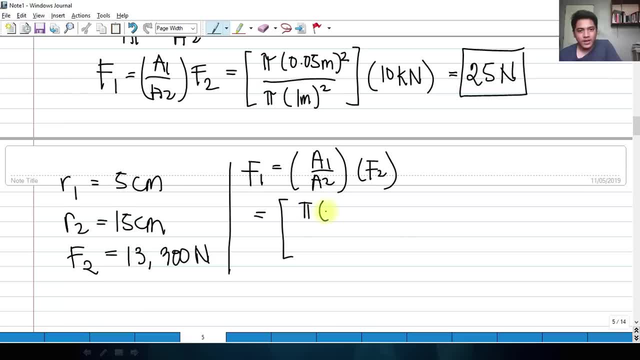 We have to convert this again into meters. So pi R1,, 0.05 meters squared over area of 2, pi over 0.15 meters squared, And that should be multiplied by the force to 13,300 N. That is the weight of the car. 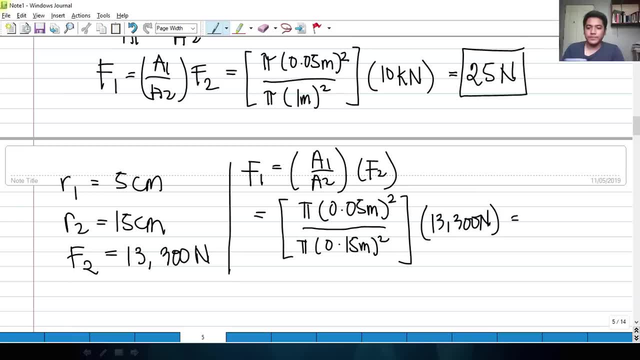 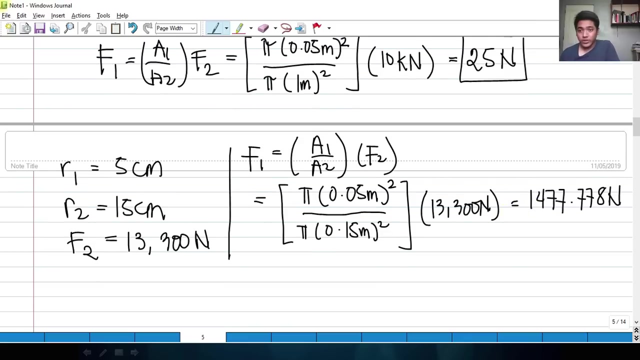 0.05 squared, 0.15 squared multiplied by 13,300.. And that should be equal to 147.778 N. Let's round it up at two, three decimals. Okay, So that is the amount of force that is needed in order to lift the car in a car lifting service station. 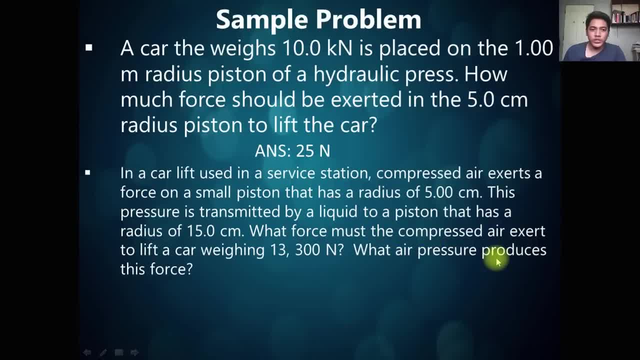 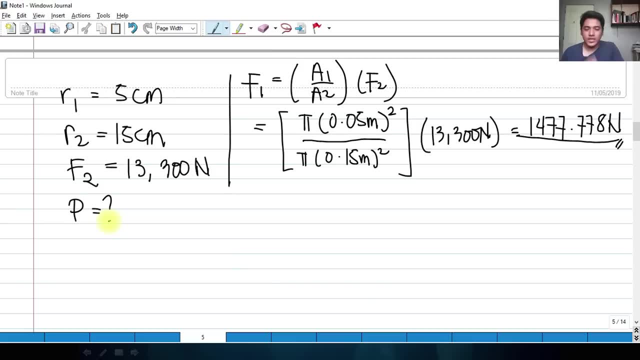 So number two: the question is actually what air pressure produces this force. So, simply, the problem is asking for us: what is the pressure? Well, since this is hydraulic press, the pressure in the left side is equal to the pressure to the right side, so that we can calculate any of the pressure. 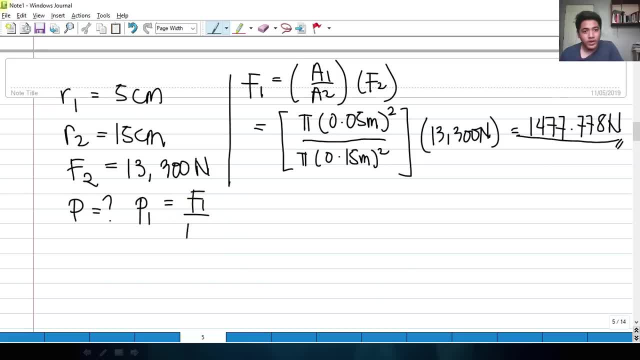 Let's say pressure 1 is equal to F1 over A1.. And our F1 is basically what we have computed here: 147.778 N divided by the area 1.. Area 1 is pi 0.05 meters squared. 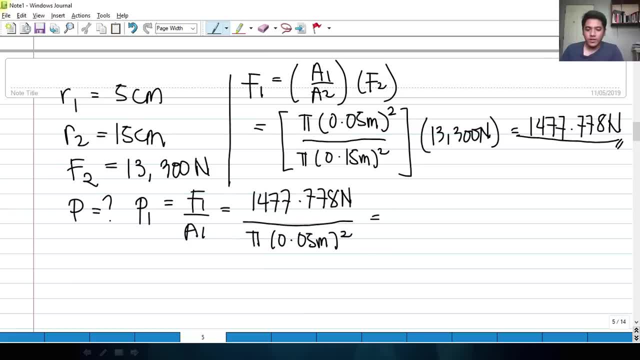 And that should result to an answer of: let's see: 188.16 times 10, raised to 3, or that is kilopascals. Okay, That is 188.16 kilopascals And for pressure 2, we have F2 over A2.. 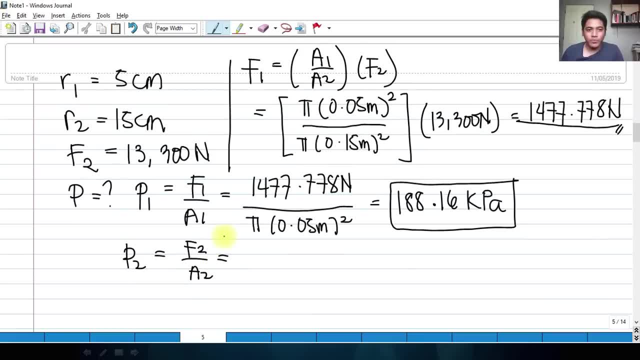 Okay, So what do we expect if we're going to compute P2?? Since this is an hydraulic press, The pressure on the left side is equal to the pressure on the right side, So these two pressures must be. Yes, you are correct. 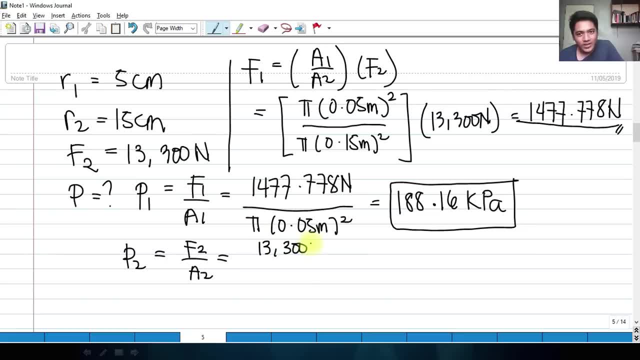 That must be equal. So we have 13,300 Newton for F2 over A2, plus is 0.15 meters squared. Okay. So 13,300 is pi times 0.15 squared. That is also equal to 188.16.. 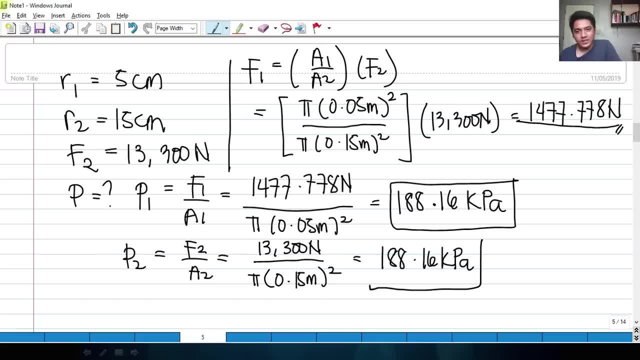 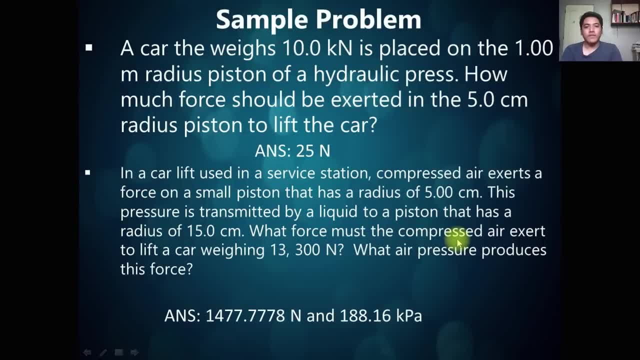 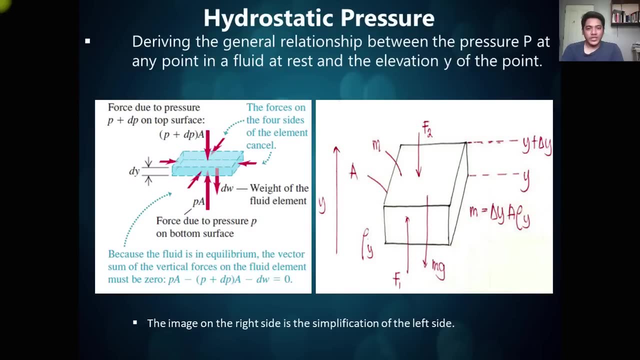 188.16 kilopascals. Okay, So that, because that works on the principle of the pascals or principle So hydrostatic pressure. So we are going to derive the hydrostatic pressure for this video And we're going to actually verify. 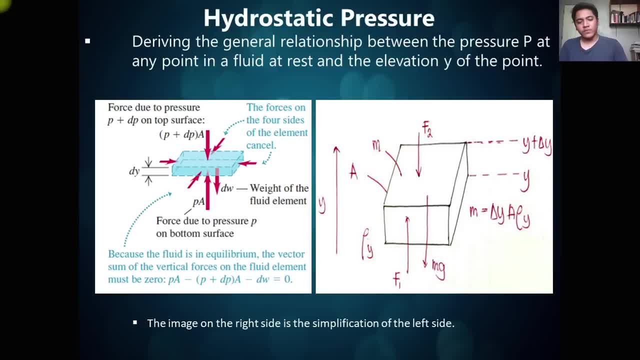 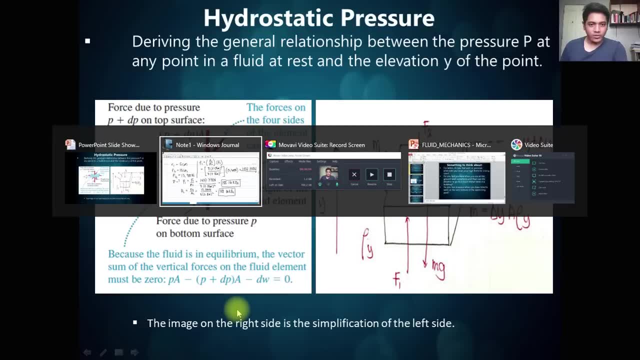 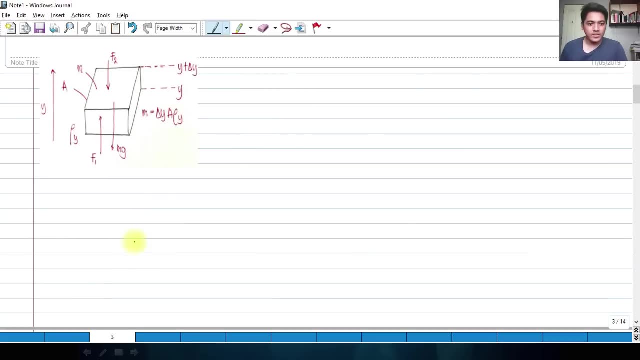 If the change in height as we go deeper into the fluid actually affects the pressure. Okay, So I would like you to consider and to listen very carefully. Okay, In this discussion, For example, class, we have this figure. Okay, So, for example, I have an open tank. 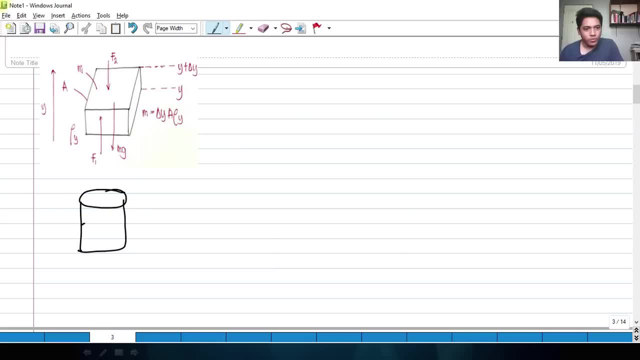 And this open tank is actually what Filled with water And I get a small amount of, let's say, a cubic size of water here. Okay, That water is sitting still doing nothing, And if I'm going to magnify this cube that, I get a portion of small portion of water. 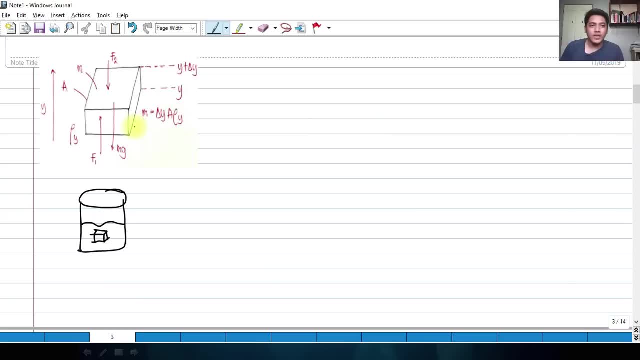 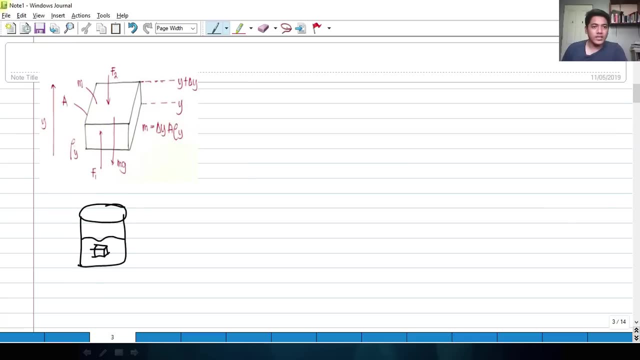 a cube portion of water. we're going to zoom it in. This is the figure. Okay, I hope you understand what I'm talking about. If we're going to look at this figure class. if we're going to look at this figure- okay. 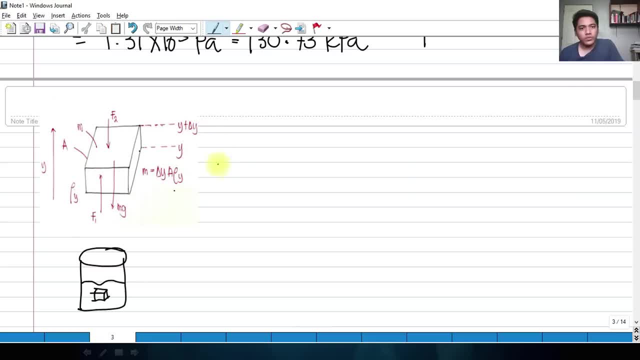 what will happen? class is that, according to our discussion, we have pressure is equal to F over A And if we're going to manipulate the equation, we have the force is equal to, due to pressure, PA. So at the very bottom of the cube, of the small cube water, okay, we have a force F1. 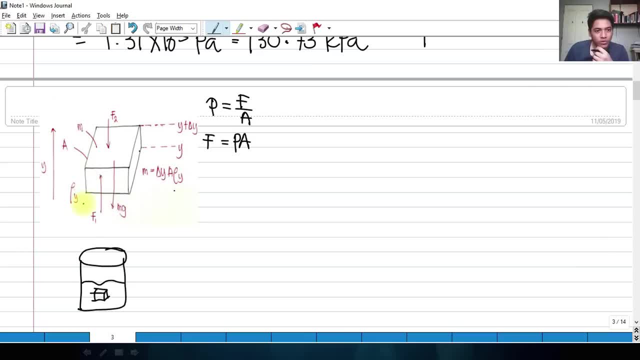 acting on the very bottom- Okay, That is called the F1 here- And at the very top of the cube, the small element, water, water element that we got here is. we have also force 2.. Okay, And of course this F is actually at height Y. 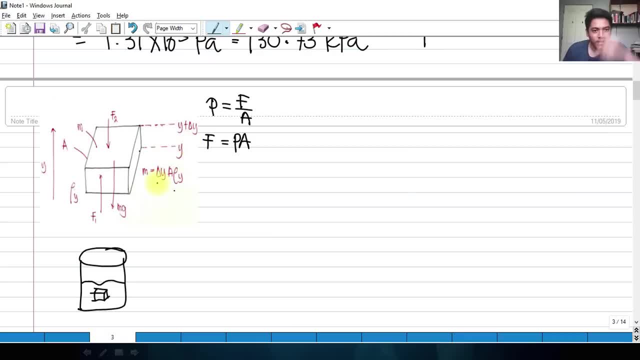 Let's label that as height Y. the very bottom of the cube, height Y, And the top where the F2 is being experienced. let's call that Y plus delta Y, Okay, So that the height is become now what Delta Y. 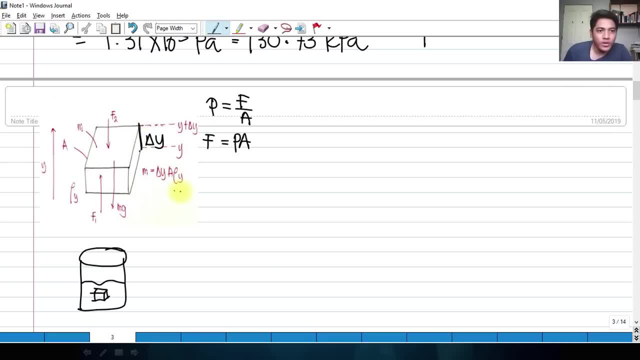 This height becomes the delta Y. Okay, So what are we going to do? class is well, of course, since force is acting perpendicularly to that water, or cube of water, small element of water, well, we must have also a force. 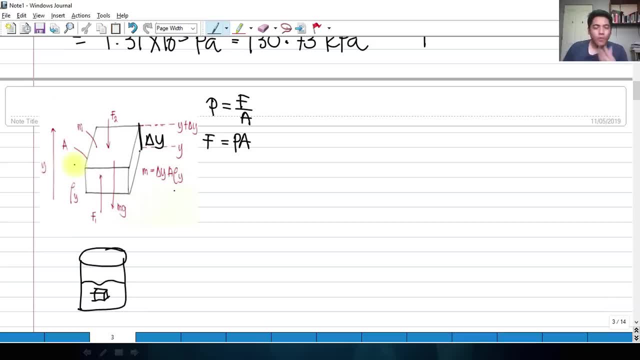 acting on the sides. Correct, But what happens is that if we have a force acting on the sides, If we have a force acting here on the side, there is also a force acting here on the other side, so that it is perpendicular to the surface of the cube. 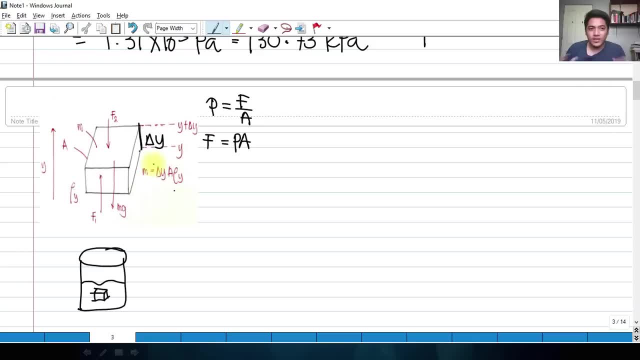 But these two forces cancel each other, So we need not to include that, Sir. but why do we have to consider the forces acting on the horizontal or in the Y-axis? Those things those forces will never cancel, because this water element, this element, that 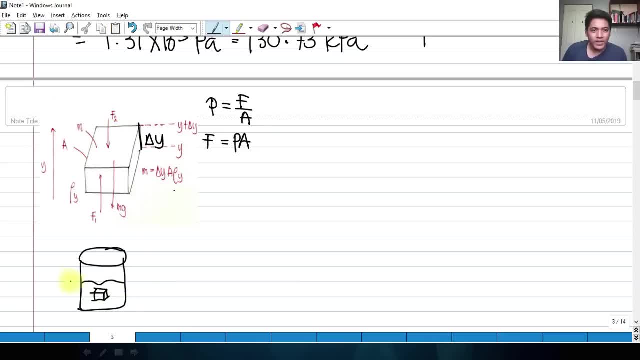 we got on this On this open tank is actually has a weight, That is what we call the mg, So that if we're going to get the summation, okay, we're going to get the summation of forces along Y. that should be equal to zero, because this fluid element is static, not. 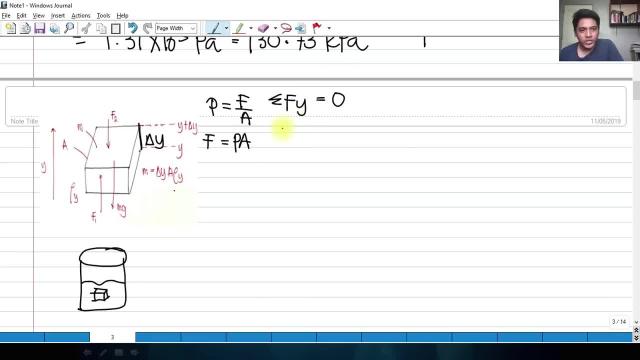 moving Okay, So that if we're going to get the summation of forces along Y, positive going upward, we have F1.. Negative going downward, we have F2. That is minus mg, So that these two, F1, F2, will never cancel because of the presence of the weight and 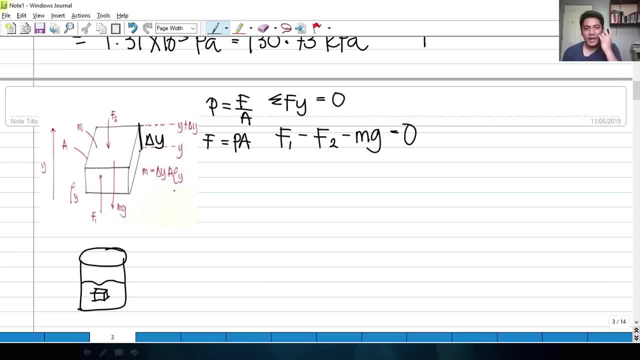 that should be equal to zero. Okay, So if we're going to, this is a cube, by the way, this is a cube, So the surface or the faces of the cube are all squares and they are all equal. Okay, So if we're going to manipulate this, force F1 and F2 to convert this, okay. 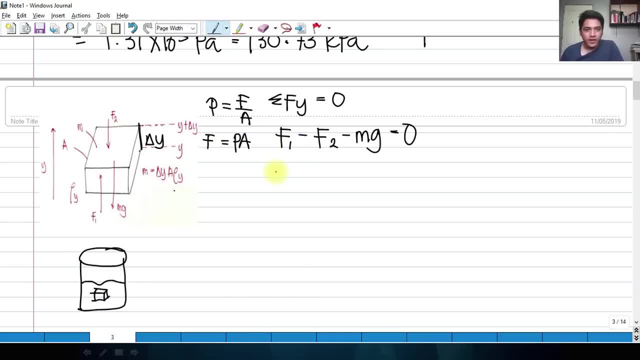 So this F1 is also equal to PA. Okay, So we have to include the A, That is, the area of the faces of the cube, that we call that A. Okay, And this F1, or the pressure, is actually yung sa F1.. 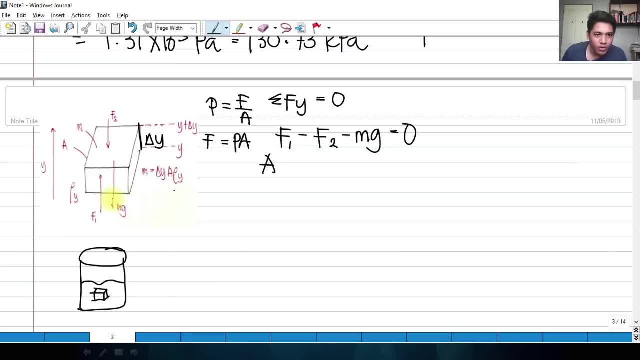 F1 is at the bottom force at the bottom of the element. So we have to what Include this at the pressure at the height Y? Why? Because it is at the very bottom and our height there we designate as y Minus. again, the area is the same for all cubes. 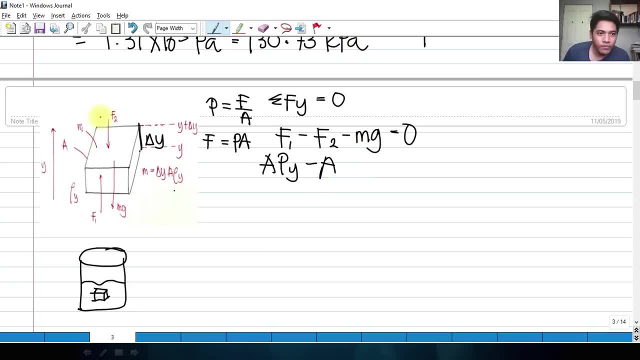 Okay, Then we have F2, the force at the very top, that is what we call the y plus delta y. Okay, That is the height. So we have to have P, the pressure, at P, y plus delta y at the very top of the liquid. 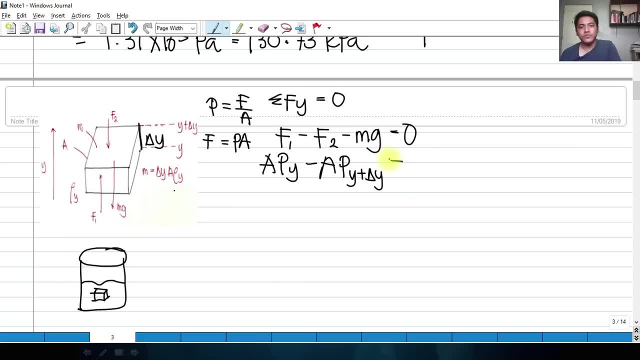 element, Okay, Minus Mg. So we have to convert M as delta y times A times the density Because, as we are going to recall, rho is equal to mass over volume And, if we are going to manipulate this, mass is equal to volume times density. 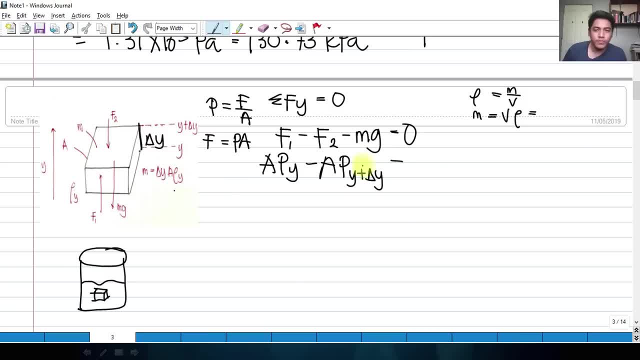 And in this case, to get the volume of this cube, simply we have to multiply the area- Okay, The area Area of the base times, height, Okay, And the height we have considered as delta, y, And of course we have to include the density of that material. 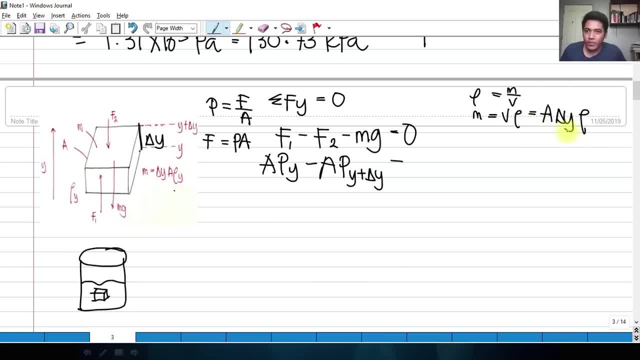 Okay, So this term A times delta y is the volume and this rho is the density, So that we are going to replace that by our M with A delta y rho multiplied by, of course, the g is equal to zero. Okay, 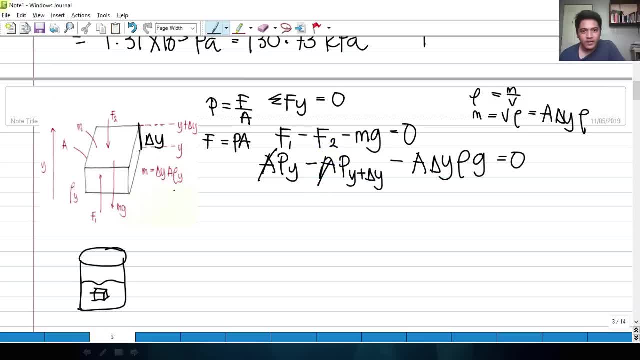 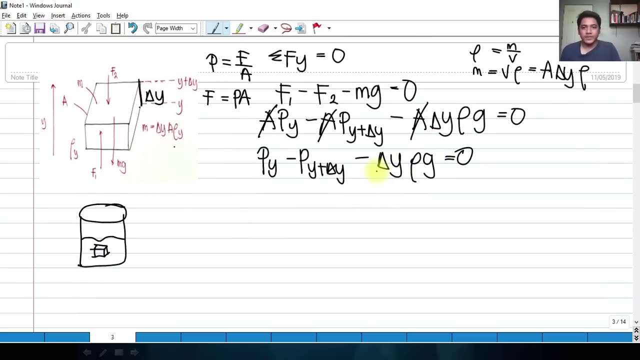 Now we can cancel what The areas here. Okay, To look this clean. So we have P y minus P y plus delta y minus delta y, rho g is equal to zero And if we are going to rearrange this equation, okay, rearrange this equation, I'm going to. 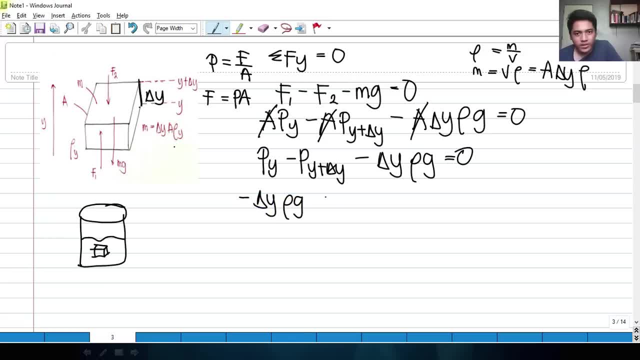 rearrange it. Negative delta y- rho g. Okay, That is equal to what Positive P y plus delta y minus P y? And if we are going to divide this both sides by, or multiply this by one over delta y, what will happen is we have negative rho g here on the left side. 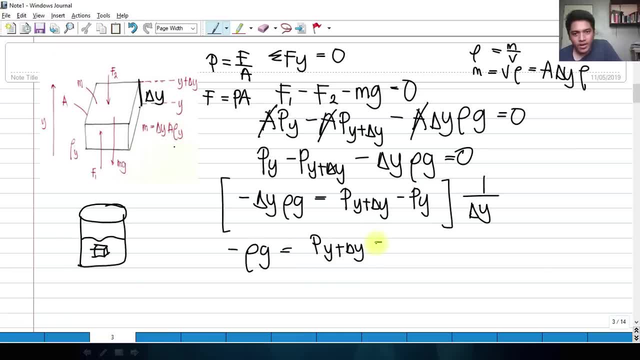 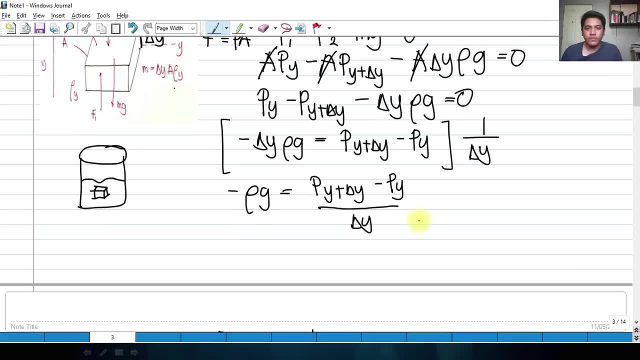 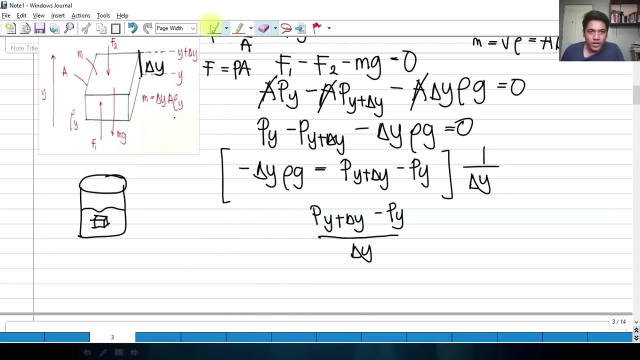 So we have P y plus delta y minus P y over delta y. Okay, So, and again, if we are going to take the limits of both sides, For example, let me just rewrite this: Okay, We're going to derive the to get the limits of both sides. 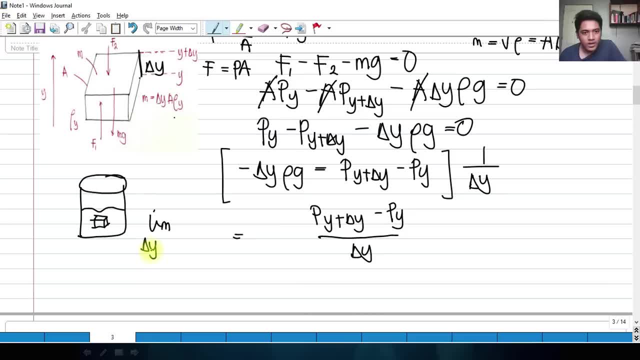 So the limit of delta y as delta y approaches zero, the limit of negative rho g, and we have to apply here the limit of P y plus delta y minus P y divided by delta y as delta y approaches zero. Let us recall that this is the definition of, basically, the derivative. 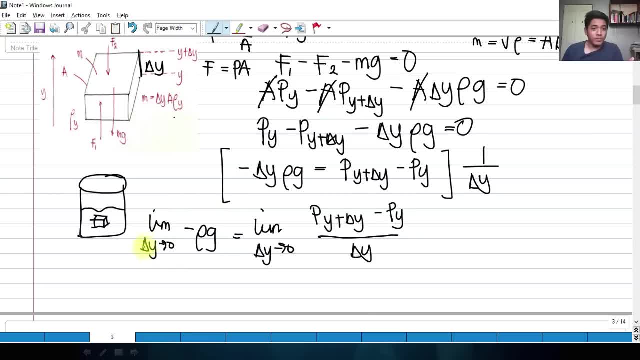 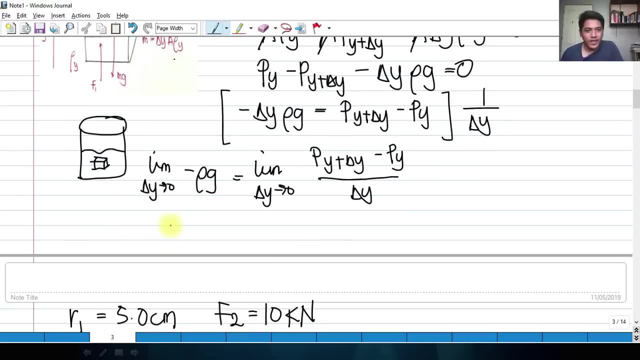 Okay So, and if we evaluate the limit of this, it's delta y, no delta y here. then this should be constant. So what will happen is that we have now negative rho g is equal to what The derivative of pressure with respect to delta y. 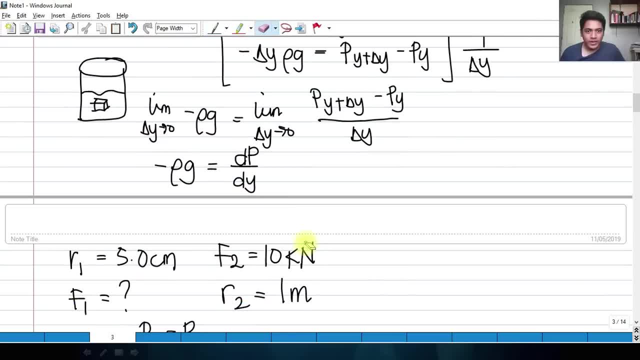 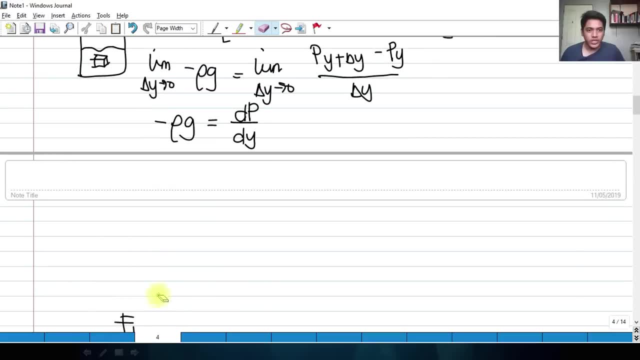 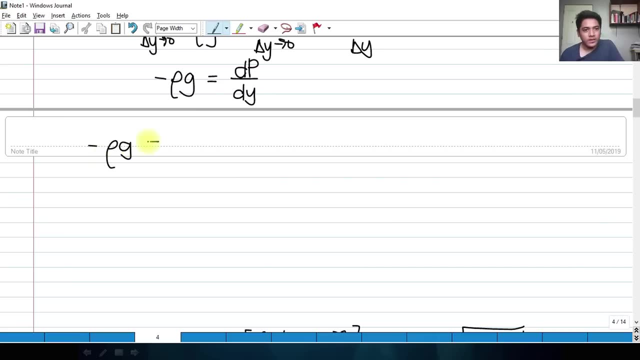 Okay, So that what will happen here, class, is that let's continue. Let me just erase this. So we have now the rho g. negative rho g is equal to dp dy. So let me just rewrite: Negative rho g is equal to dp change in pressure with respect to y. 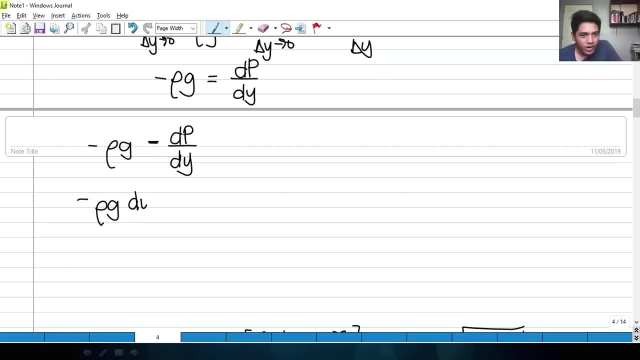 We're going to cross multiply this negative rho, g, dy is equal to dp. And if we're going to integrate these two- okay, integrating this from P1 to P2,, integrating this from height 1 to height 2, what will happen? 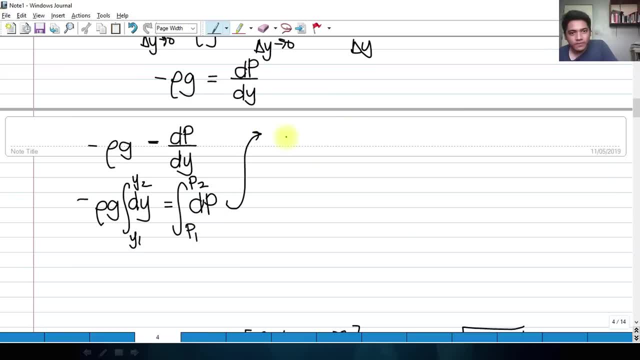 We have a definite integral, So it is easy to evaluate definite integral. we have The integral of dy is y and that is evaluating limits from y1 to y2.. And the integral of dp is simply P, evaluating limits from P1 to P2.. 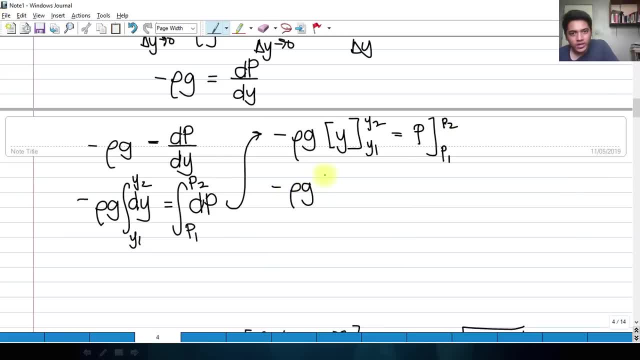 So what will happen is that negative rho g is now equal to y sub 2 minus dp, So y sub 2 minus y sub 1, and equal to P sub 2 minus P sub 1.. And if I'm going to multiply this all by negative 1, what do I have to get is, let's say, rho. 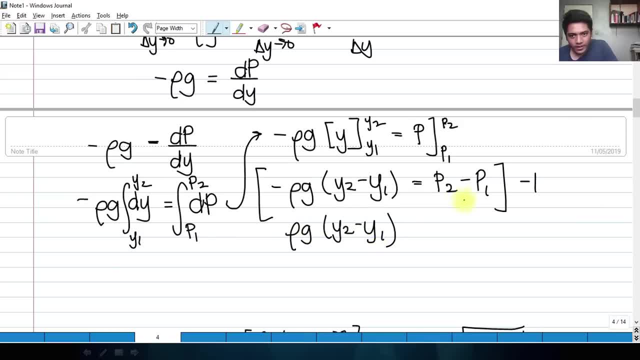 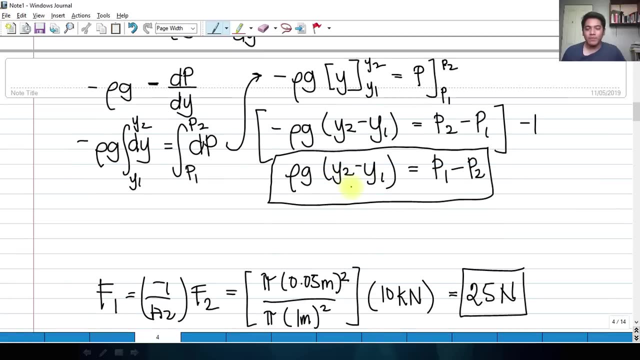 g times y2 minus y1 is equal to P1 minus P2.. Now this is the hydrostatic, or the change in pressure whenever we change our height. Okay, So this y2 and y1 can be replaced as height 2 minus height 1.. 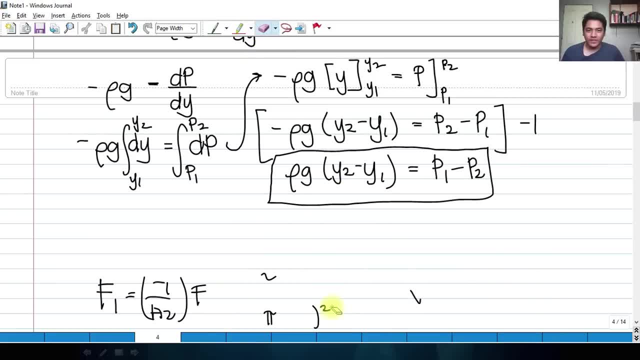 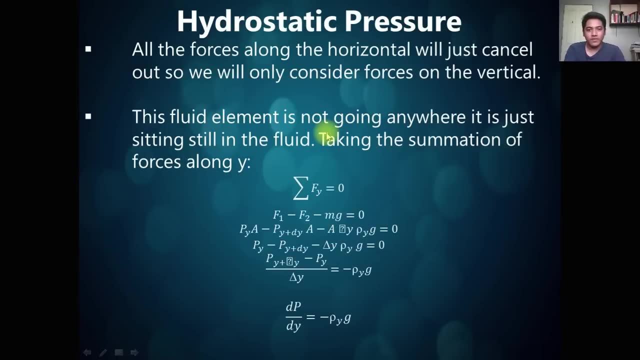 Okay, Because we are dealing with the height. Okay. So we have proven that as we go on deeper, there is a pressure change because of the change in height. Okay, So that is our formula, So I have derived it here, Okay. 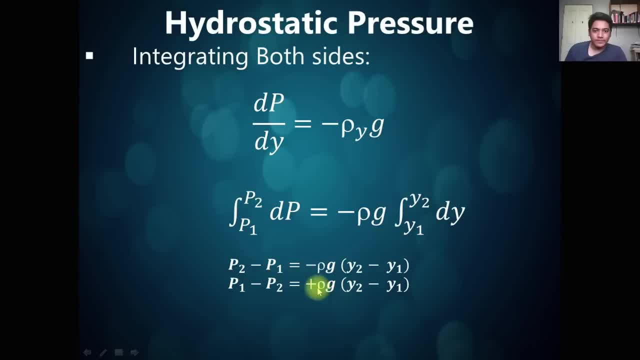 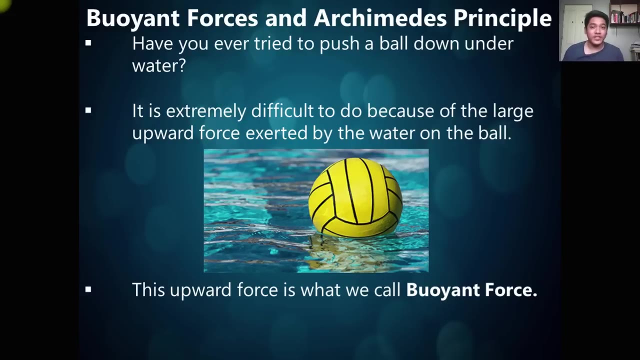 So now we have gotten this formula. Okay, So there is a change in pressure whenever there is a change in height. Okay, So to continue our discussion, we're going to talk about the Boolean forces and Archimedes principle, on the latter part of our study in fluid mechanics. 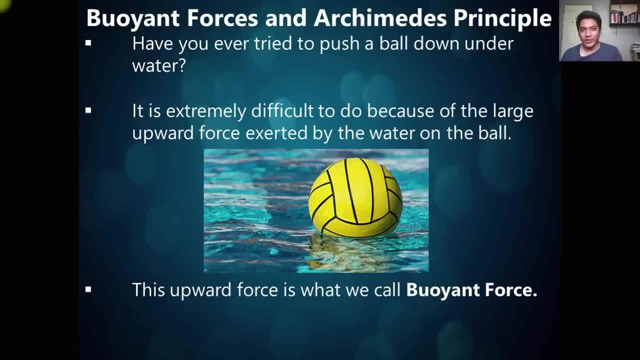 So have you ever tried to push a boat down underwater? Well, it's very hard to do because there is actually what we call the Boolean force. It is extremely difficult to pull down, push down a boat underwater because of the large upward force exerted by the water on the boat. 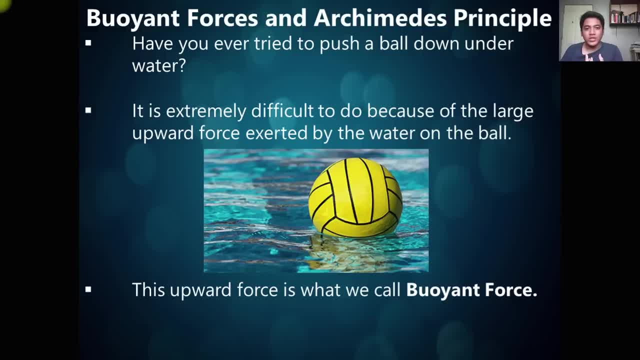 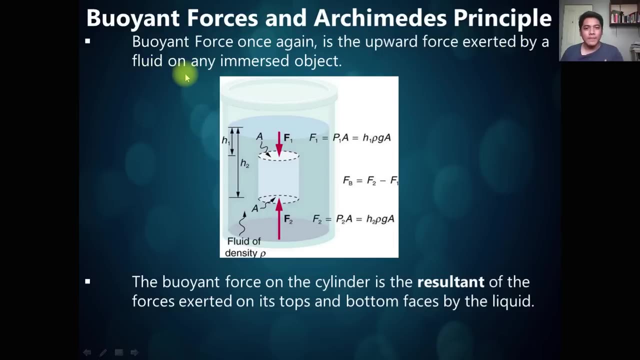 And that's what we call the Boolean force. The Boolean force is actually the force that the water or the liquid exerted on the object, any immersed object. That is what we call the Boolean force, And Boolean force, once again, is the upward force exerted by a fluid on any immersed object. 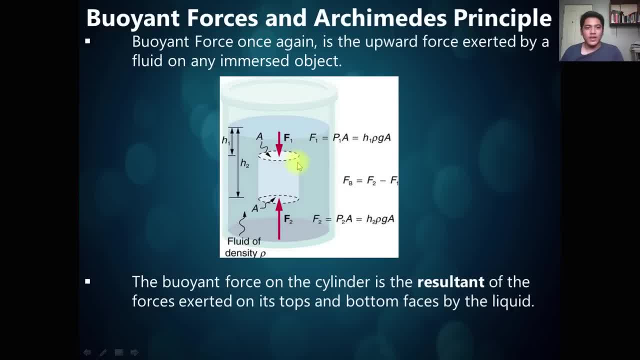 So, for example, we have a cylinder here and we have a- we made a cylindrical shape here that is being immersed on this water fluid. So we have two forces acting on its top and on its bottom, And the Boolean force, by formula, is actually the magnitude or the resultant of the forces. 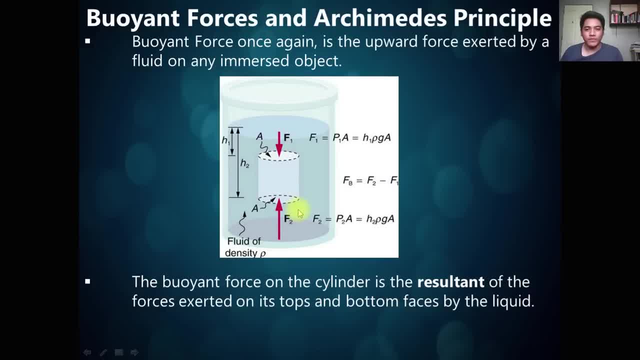 exerted on the top and the bottom of the phases of the liquid. So, in other words, FB is equal to F1.. Okay, F1 or F2 minus F1.. The resultant of the forces acting on the top and on the bottom of the object. 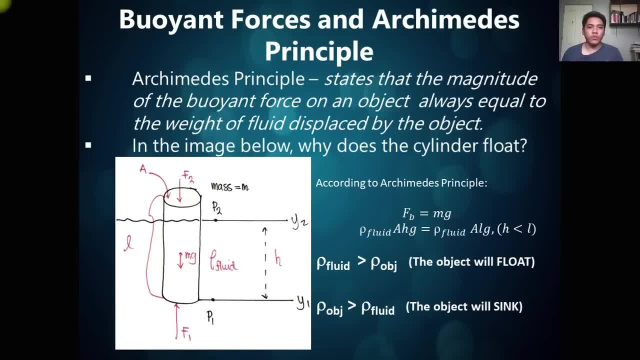 Okay, And we have the Archimedes principle. Archimedes principle only states that the magnitude of the Boolean force on an object by the liquid is always equal to the weight of the fluid displaced by the object. So we have here the formula according to Archimedes principle. 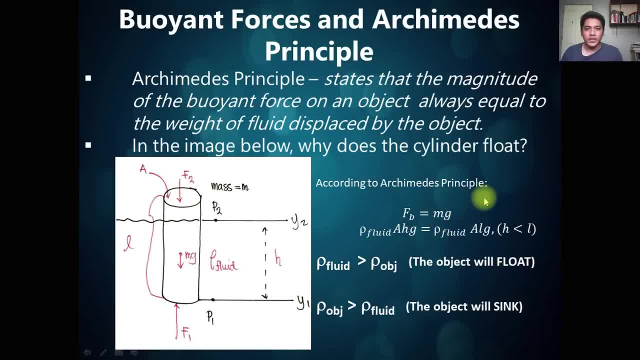 We have the Boolean force is equal to the magnitude of the Boolean force, equal to the weight of the fluid displaced. Okay, So, let's take note of this. This is an important concept or principle, Okay, So, as I've said a while ago in the video, what if we have the determining factor? whether 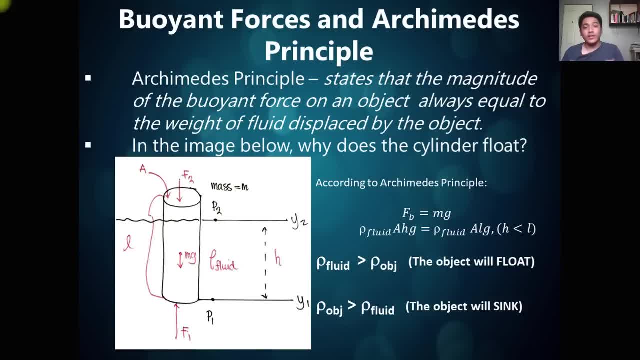 the object will float or sink when it is submerged into a liquid. is that its density? So here is the determining factor. If the density of the fluid is greater than the density of the object, then the object will float. Okay, Regardless of their size, regardless of their weight. 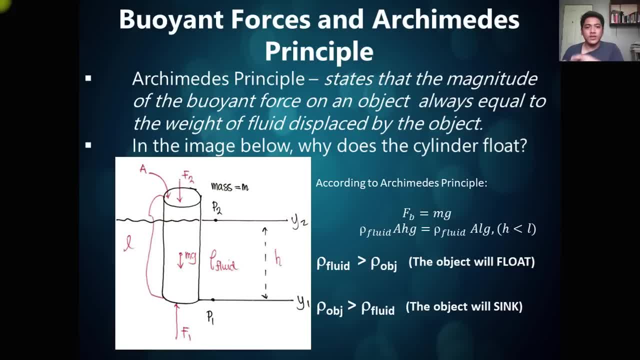 As long as the density of the fluid is greater than the density of the object, the object will float. On the other hand, if the density of the object is greater than the density of the fluid to which it is immersed, the object will sink. 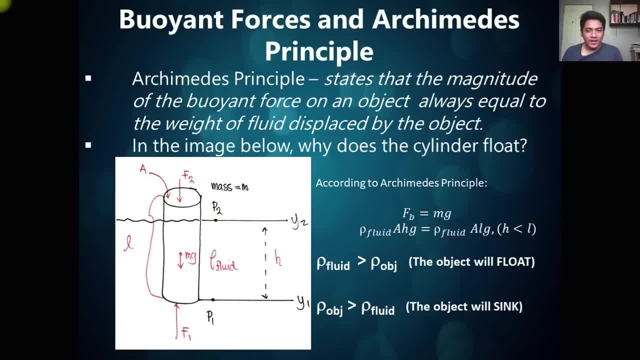 So our grandfather would actually joke something about us Which is Much massive. Okay, Is it the one peso coin or the ship? Okay, If you answer the ship, why does the one peso coin sink and the ship not, If it is much massive than the one peso coin? 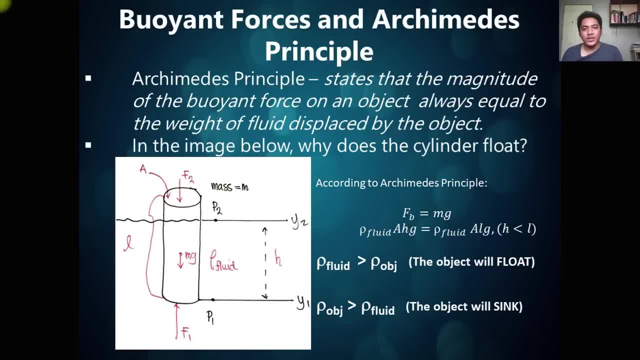 Okay, Because the one peso coin is actually has a greater density than the density of the fluid or the water. Okay, So the one peso coin always sink And the ship will actually, by convention or without any large amount of waves. well, technically, that ship is made of wood and the density of wood is greater than the density. 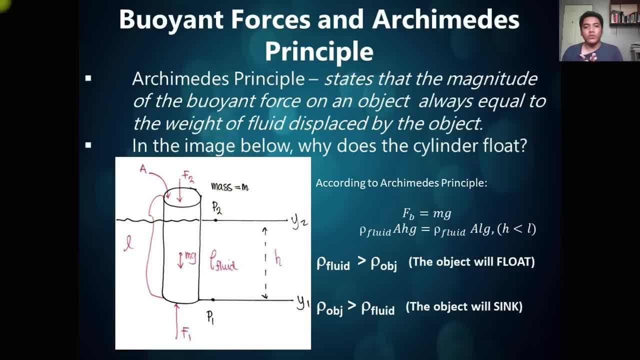 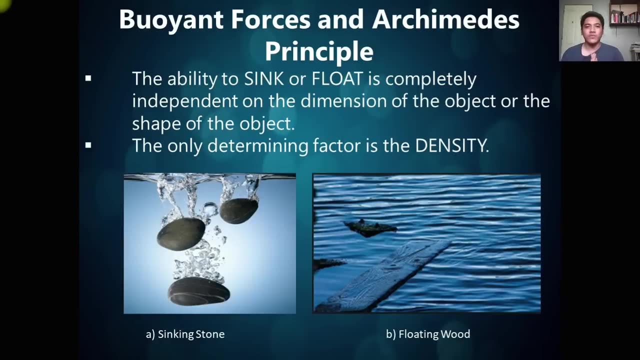 of the fluid or the sea water, then we can conclude that that ship would actually float. Okay, So the only determining factor whether the object will sink or will float is the density. Okay, So the ability to sink or float is completely independent on the dimension of the object. 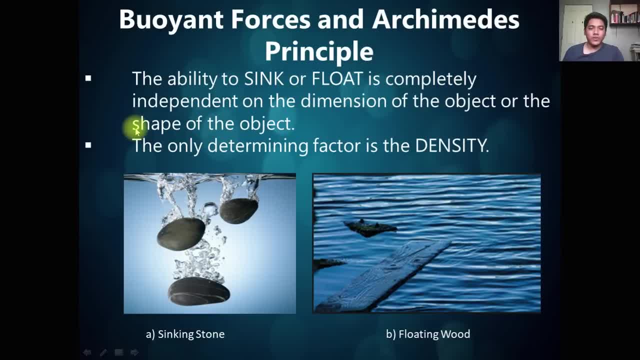 or the shape of the object. The only determining factor is the density. So we have here, for the first image, the sinking stone. We can conclude that the density of this stone is greater than the density of the water to which it is being immersed. 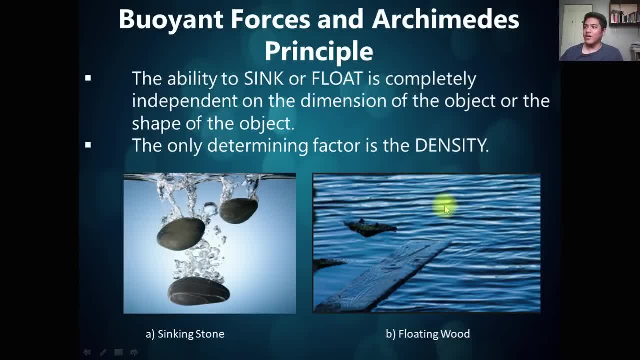 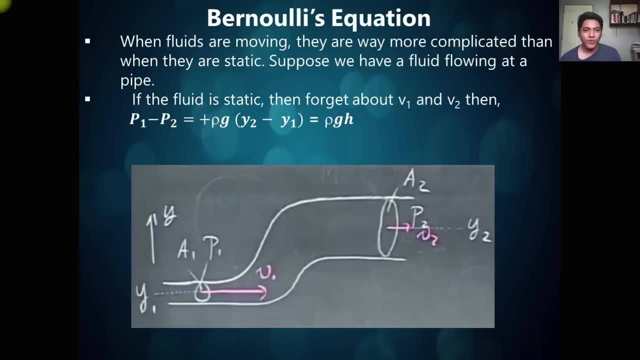 And we have the floating wood. regardless of their size, regardless of their shape, Okay, So it's only determining factor whether it will float or not is the density. So we have now the Bernoulli's equation. When fluids are moving, they are way more complicated than when they are static. 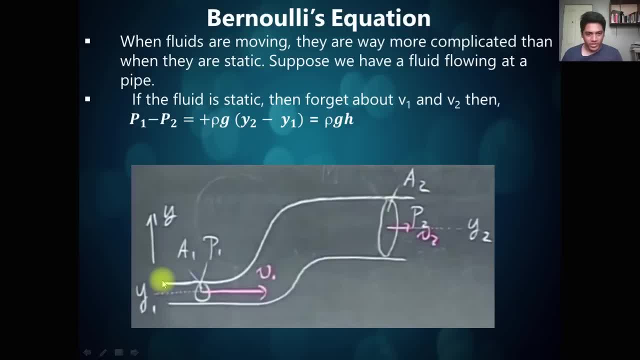 So suppose we have a fluid flowing at a pipe. This is our pipe. Okay, If the fluid is static, then forget about V1 and V2.. Okay, And forget about this hydrostatic pressure. Okay, We will no longer use that, because this formula is only for fluids that are statics. 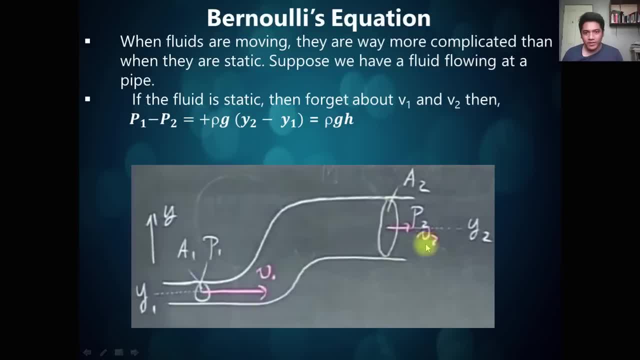 So how about if they move? For example, we have a pipe here, Okay, And this pipe is filled with fluid- I'm so sorry- So fluid, So that when the fluid flows here, it is flowing through a cross-sectional area, one, and it. 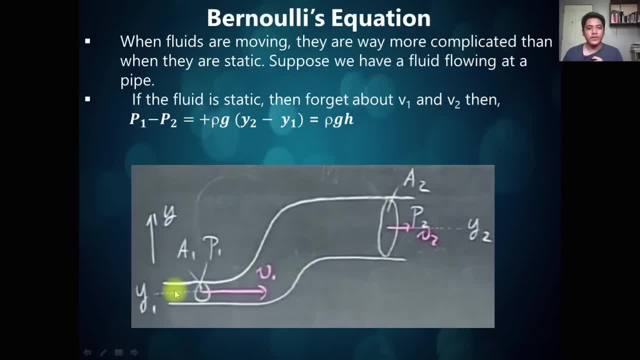 has a flow. Okay, It has a velocity V1.. So when this fluid flows here and eventually flows here, there will be a change in pressure, because actually the cross-sectional area here is not the same as the cross-sectional area here, And of course there will be a change in velocity. 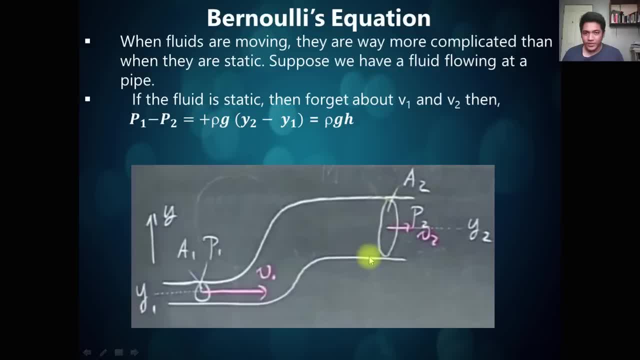 Why? Because there is also a change in the opening of the tube or the area of the tube. So we have the velocity one here and we have the velocity two here. Okay, So if we make a height of which we use this as our reference in Y1, the Y1, and we have 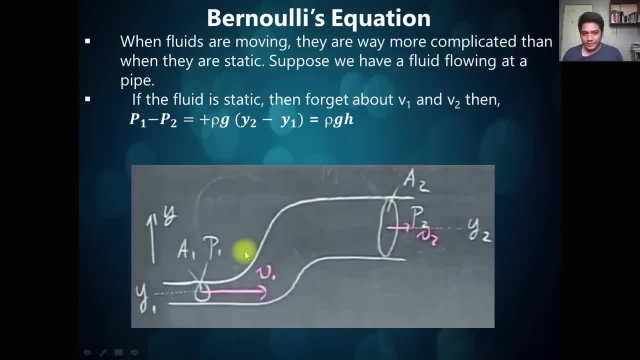 Y2 here. so there is also the presence of what? The potential energy because of the height, the velocity, kinetic energy, the presence of kinetic energy because of the velocity and of course, the presence of pressure. So in Bernoulli's equation we have three players. 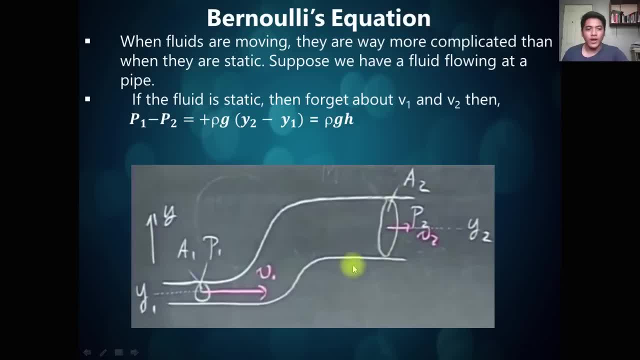 We have the potential energy, because there is a height- Y1 and Y2, and we have velocity one and velocity two, which reminds us of kinetic energy, And we have, of course, the pressure due to difference in area and the force of the fluid. 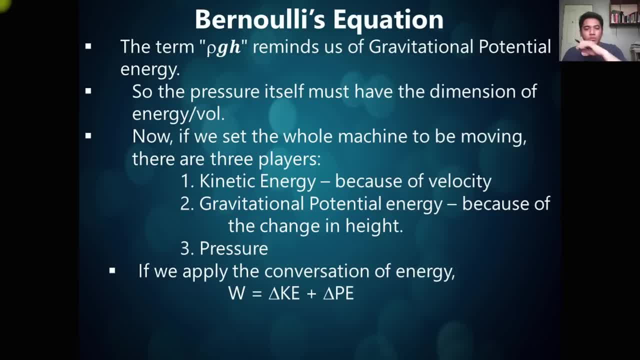 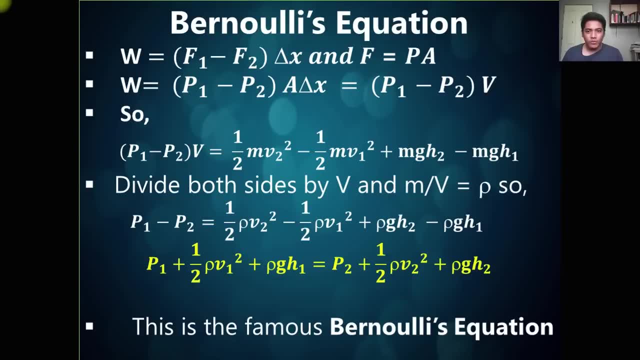 acting on that area. Okay, So I would not be really deriving you the Bernoulli's equation, because it is a tedious derivation, Okay, But rather I would like you to take note of this formula, which is the famous Bernoulli's. 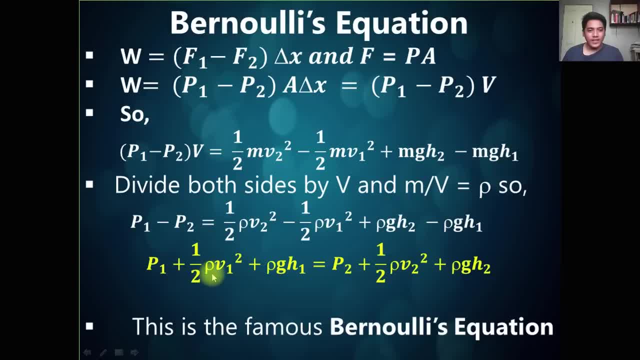 equation: We have P1 plus one, half The density of that fluid. Okay, V sub one squared, Okay The velocity. one of that first velocity of the fluid plus rho, which again is the density. G is the gravitational force And height one is the height of the tube with respect to a certain reference. 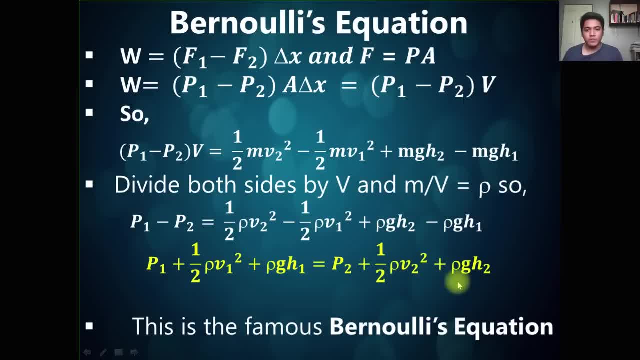 That is equal to P2 plus one half rho V sub two squared plus rho GH sub two. This is the famous Bernoulli's equation. And, of course, before we solve the, usually the problem here is solving for the velocity at the other end of the tube or the pipe. 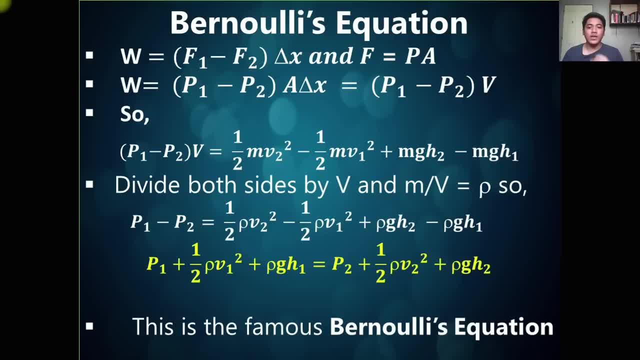 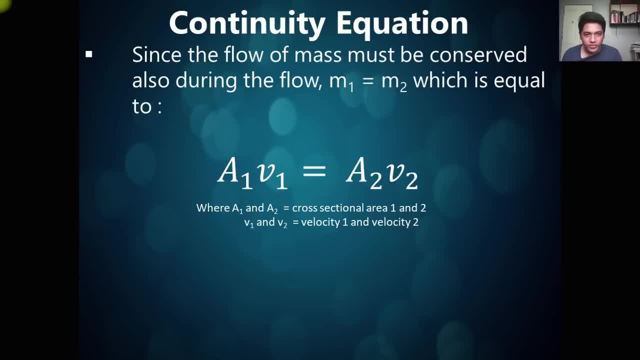 And solving the pressure. So, in other words, before we can solve the pressure, we have to take note of what we call the continuity equation. And the continuity equation is simply A1, V1, where A1 is the cross-sectional area for 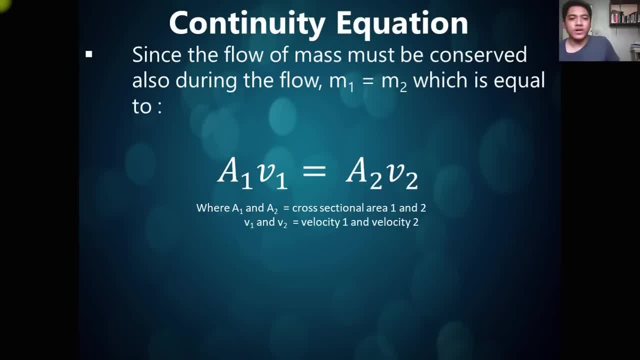 one and A2 is the cross-sectional area for two. V1 is the velocity one and the velocity two During the fluid is moving. Okay, So let's try to solve a problem about the gasolines. Okay, So let's try to solve a problem about the gasolines. 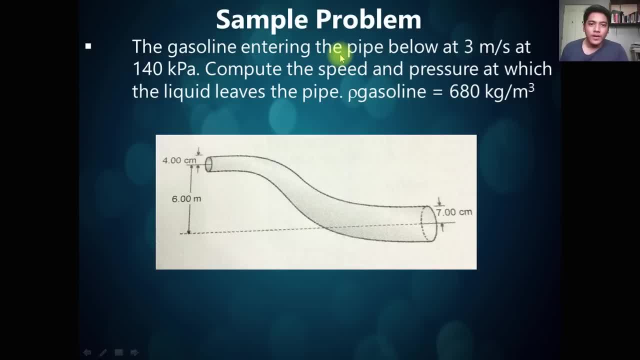 Okay. So let's try to solve a problem about the gasoline problem, The gasoline entering pipe. entering the pipe below at three meters per second, here, Okay, At 140 kilopascals, Compute the speed and pressure at which the liquid leaves the pipe. 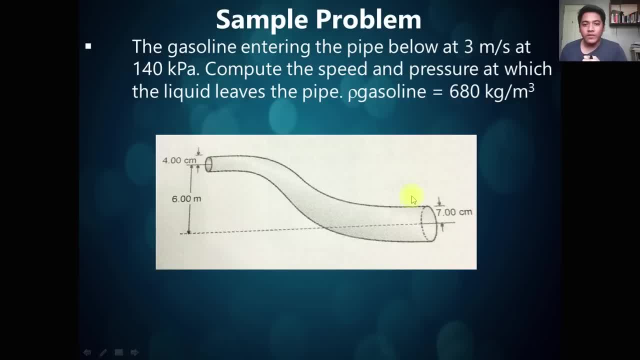 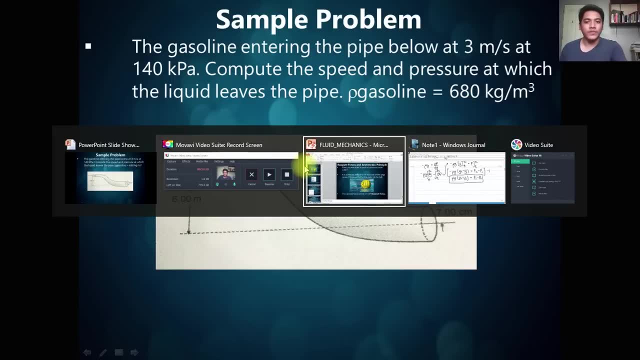 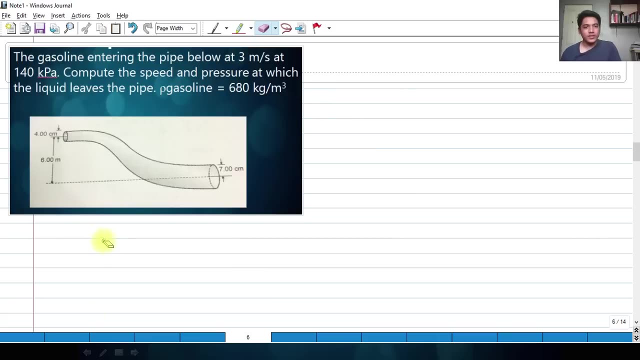 Okay, Compute the pressure and the velocity of the fluid. at this point, The density of gasoline is 680 kilogram per cubic meter, If I'm not mistaken. I have copy pasted here. Okay, Again, our formula is, if you have taken note of that, for continuity equation we have: 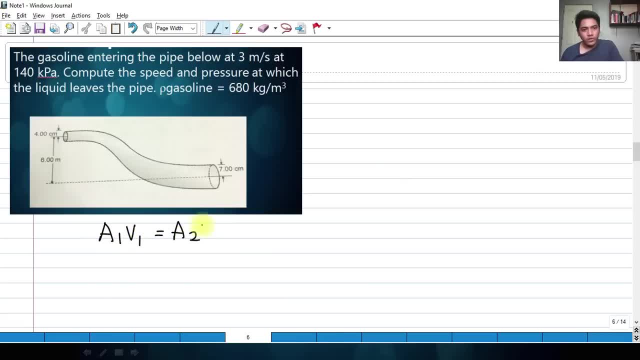 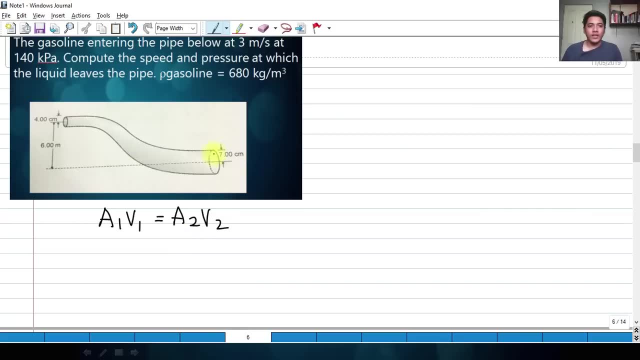 A1, V1 is equal to A2, V2.. We must use first the continuity equation to find the velocity of the fluid at that point at the second point to which it leaves the pipe. So in order for us to get V2, okay, V2 is simply equal to A1 over A2 times the velocity. 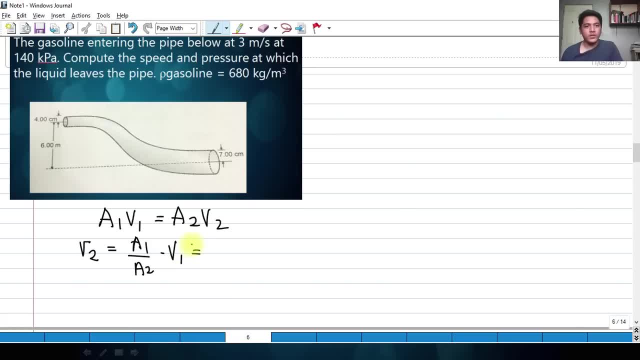 Okay, So A1 is. we can see here from the. given the radius is 4 cm, We have to convert that into meters And the pro-sectional area of the tube or the pipe is actually A. Yes, that's right. 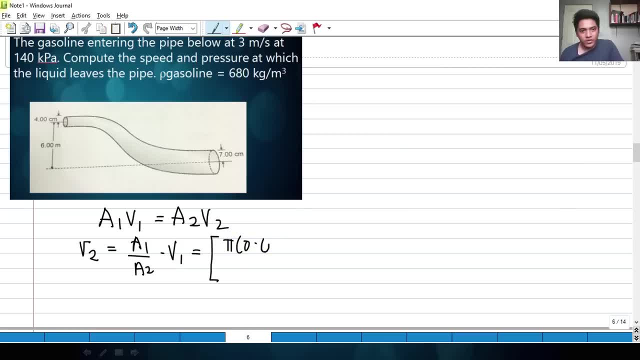 A circle- pi- 0.04 meters squared. Okay, 4 cm. 0.04 meters squared. Divided by pi, The area of the other one is 0.04 meters squared. Okay, 0.07 meters squared. 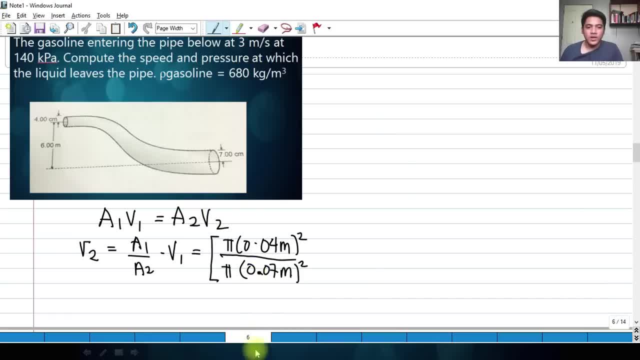 That's the radius. I'm so sorry. The area is pi times r squared: pi r squared. Okay, So we have here the formula, And multiplied by V, velocity 1.. Velocity 1 is actually what? 3 meters per second. 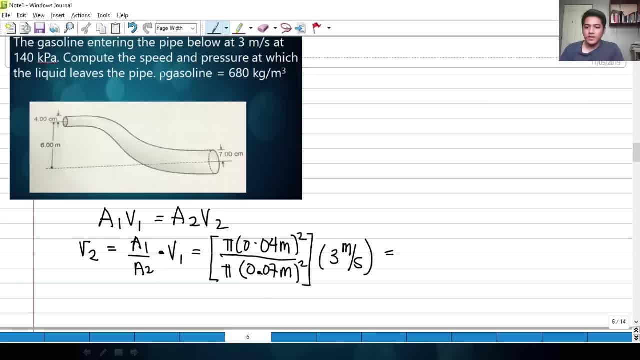 So if we're going to compute that, pi's will cancel. So we have 0.04 squared, 0.04 squared divided by 0.07 squared times 3. And that is 0.98 meters per second. So this is now our velocity 2.. 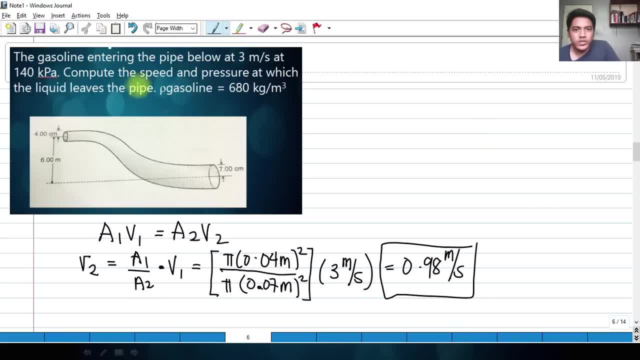 Okay, How do we find the pressure? We're going to use the Bernoulli's equation, We're in pressure. 1 plus 1 half rho V sub 1, squared plus rho gh1, is equals to p sub 2 plus 1 half rho V sub 2, squared plus rho gh sub 2.. 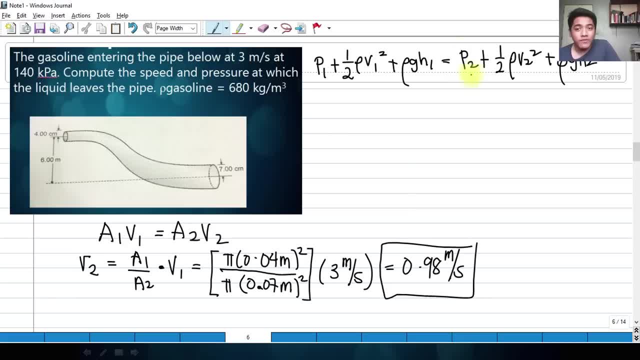 Okay, And we are after to find the p sub 2.. So we have to isolate p sub 2.. Okay, So we have p sub 1 plus 1 half rho. If we're going to factor it out, transpose this on the left side. 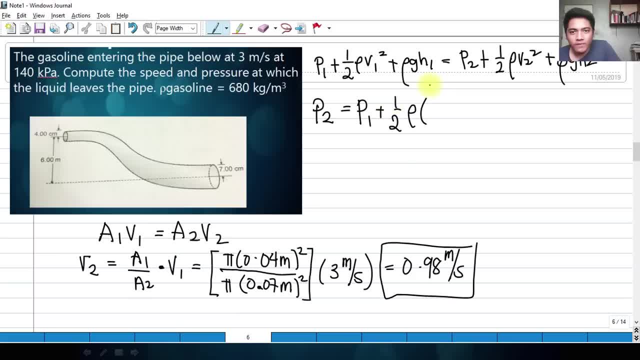 Okay, And factor out 1 half rho. Okay, 1 half rho, That should be V1.. V1 squared minus V sub 2 squared plus rho g. Okay Again, we're going to transpose this on the left side. 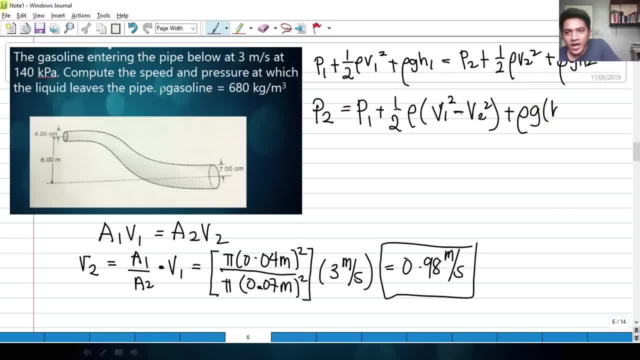 Okay, So that we can factor rho g, That is height 1 minus height 2.. So the pressure 1 is 140 kilopascals plus 1 half, The rho is 680.. That's the density of the gasoline. 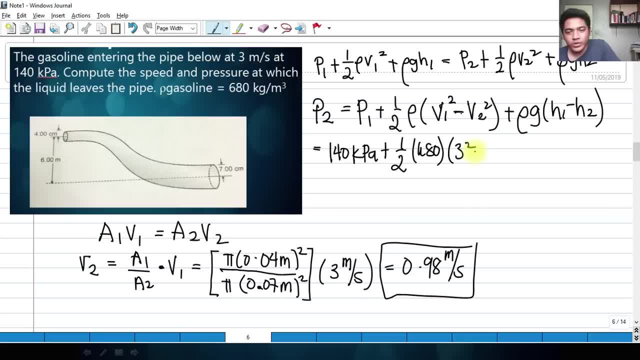 V sub 1 is 3 squared, 3 meters squared. meter per second squared. I would not write the units so that we could consume little space. So 3 squared minus 0.98 squared, plus the rho, again 680 kilograms per cubic meter times. 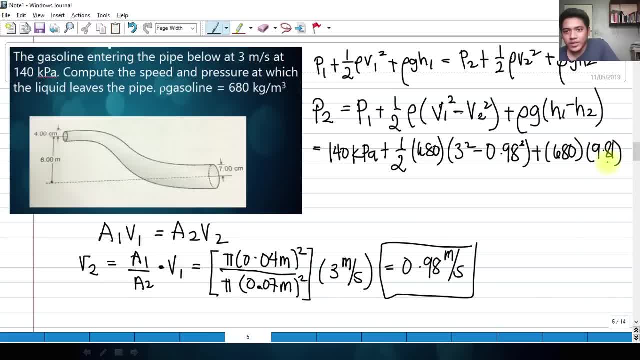 the g, That is 9.81 meter per second squared multiplied by height 1 minus height 2.. And according to our figure, height 1 is 6 meters. Okay, The reference is the height 2 is 0.. So 6 minus 0 or simply 6.. 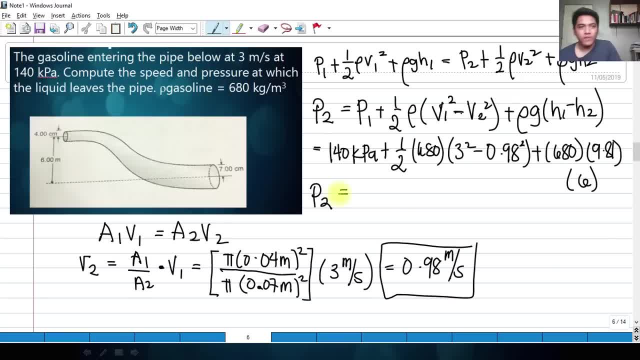 So we're going to compute the pressure 2 of that. Okay, Let's try to compute 140 kilopascals plus 1 half 680 times 3 squared minus 6.. Okay, 0.98 squared plus 680 times 9.81 times 6.. 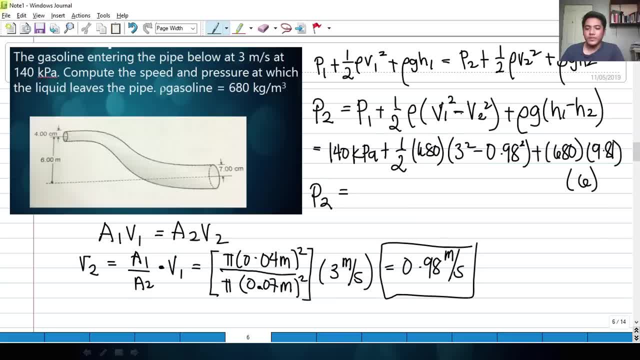 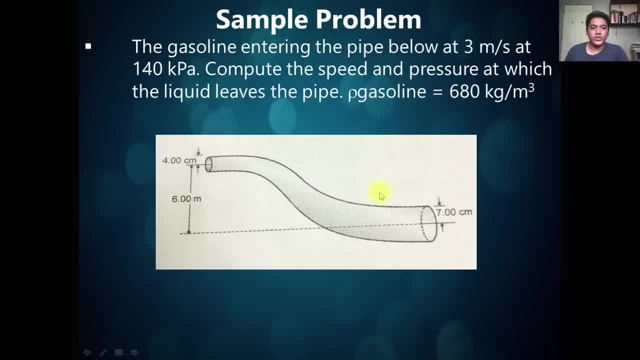 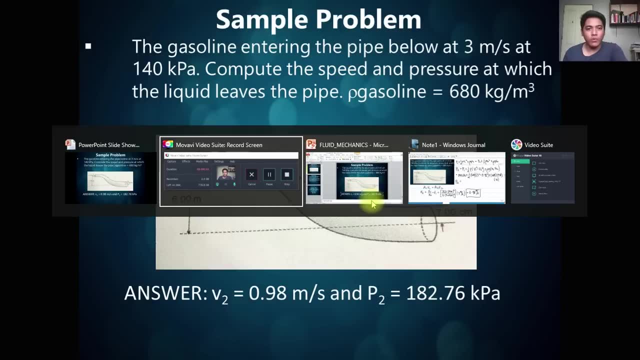 And that is 182 or 183.. Oops, So our answer should be 1. 182.76 kilopascals, 182.76 kilopascals, 182.76 kilopascals. So that's all. 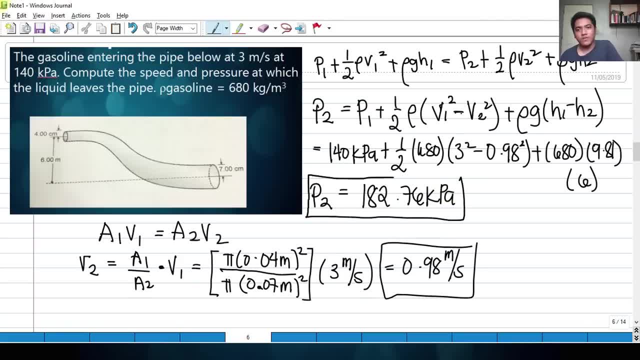 Okay, So thank you so much for listening. Here are our references: University Physics by Sir Wei and Modern Physics, University Physics by Young and Friedman, and Physics book by Gary B Conrado. That is a Filipino author. So thank you so much for listening and God bless you. 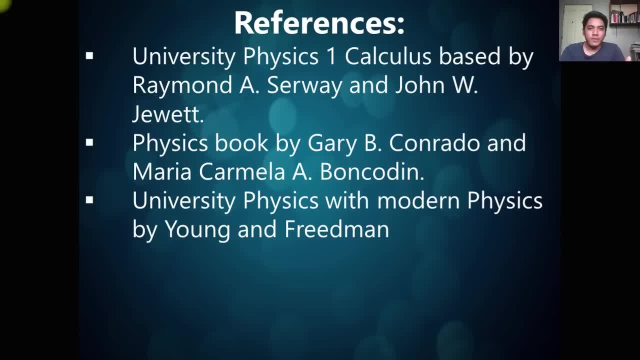